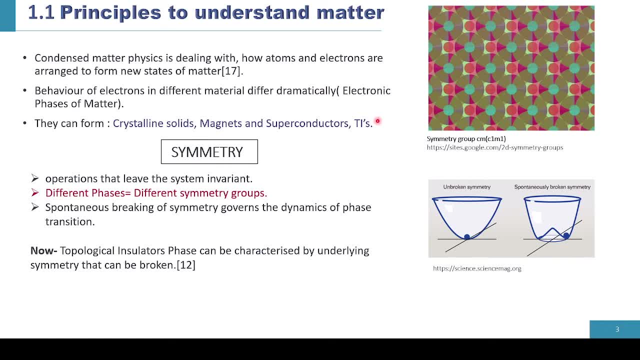 like our superconductors and topological insulators. So symmetry is one of the things that we need to understand in order to understand the matter. So symmetrical operations should leave the system invariant and different symmetry groups will create different phases of matter and a new phase change can happen when spontaneous symmetry breaking happens. So there are different. 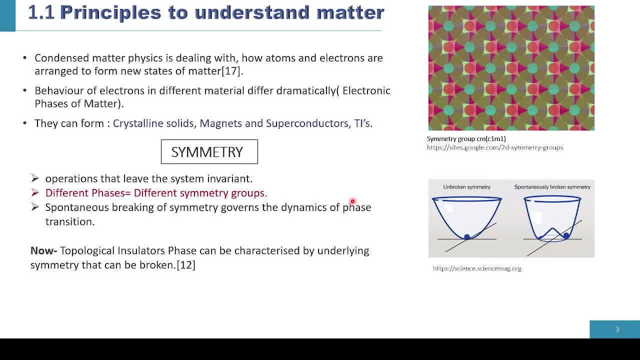 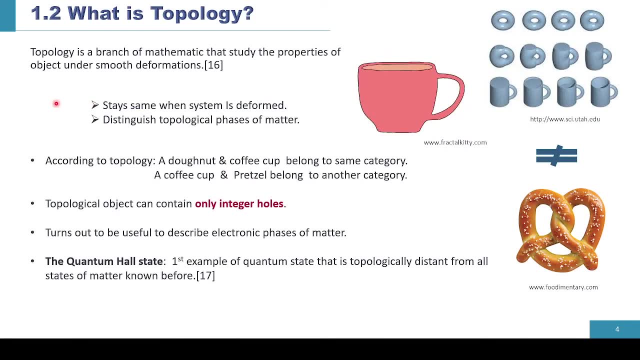 types of symmetry. We have the rotational symmetry, translational symmetry, time reversal symmetry and so on. So now, what is topology? Topology is nothing but actually a branch of mathematics which study the property of an object under adiabatic deformations. So, according to topology, a donut and a cup belongs. 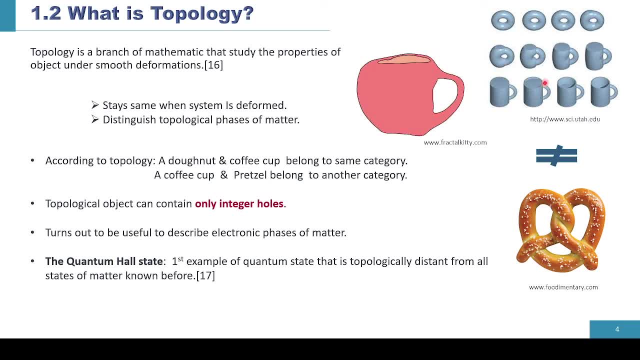 to same category, but a donut and a pretzel belongs to different category, and why it is so? The answer is very simple: A donut and a cup have same single holes, while the other half is different. So this is a simple idea. 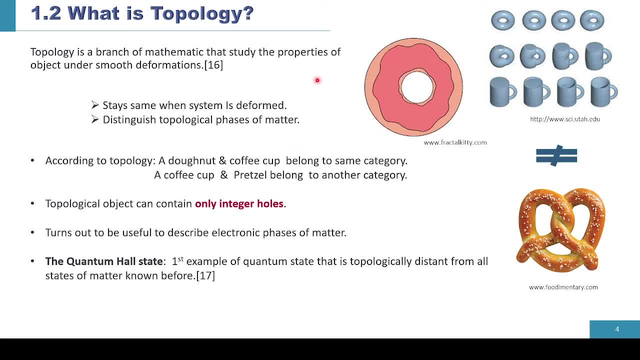 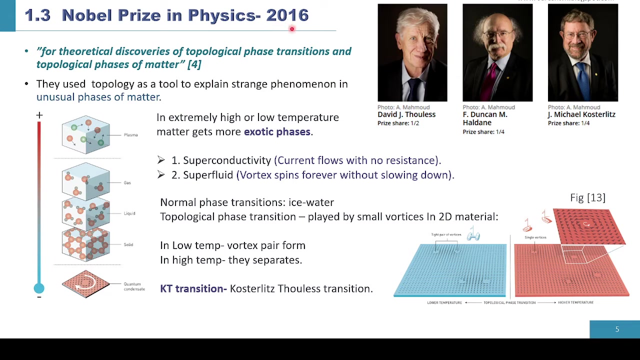 Here in topology, we can only have integral holes, and this simple understanding came up to be a very good thing to describe the electronic phases of matter, And the quantum hard state became the first example of topological distinct matter from other types of phases. The Nobel Prize in Physics for 2016 was actually awarded to Professor Tholes, Halty and Koster. 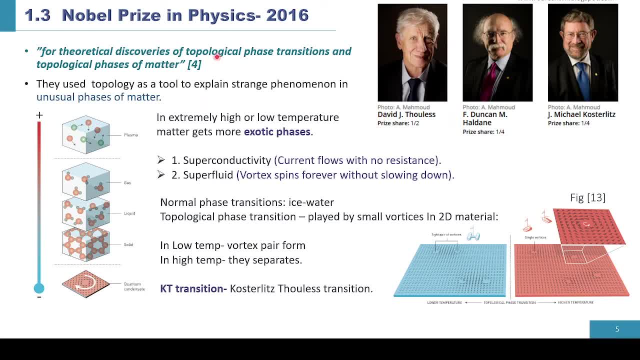 for their theoretical discoveries of topological phase transitions and topological phases of matter. They used this topology as a tool to explain the phenomena of unusual, exotic material phases. you know, matter behave drastically, dramatically higher temperature and low temperature, especially in the low temperature, and they can create exotic matters like superconductivity and 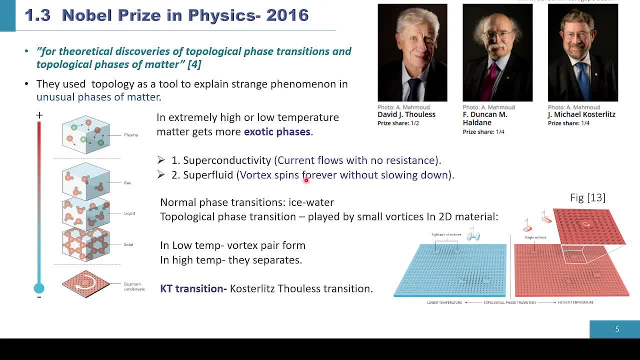 superfluid. in superfluid, just the vortex, spin vortex formation happens and they can just spin forever. so in high, low temperature the spin vortex forms as pair and then in high temperature they get separated and this transition is called constant Thouless transition. but we are not going to go into this. 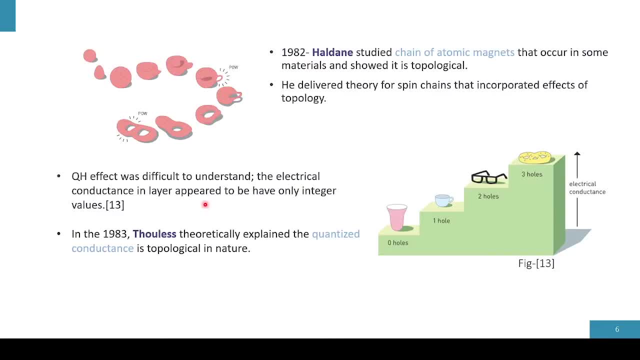 because this is just regarding the novel price. then in 1982 professor Halliday actually studied the topological aspects of atomic magnet. now, for our understanding from this presentation, we have to focus on professor Thouless. he in 1983 actually gave a good explanation to for why the, the hollow conductance, is quantized. 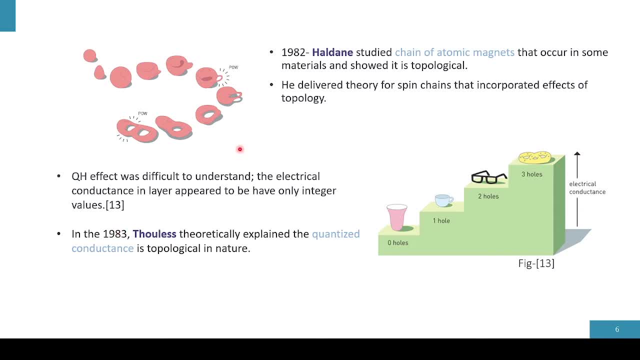 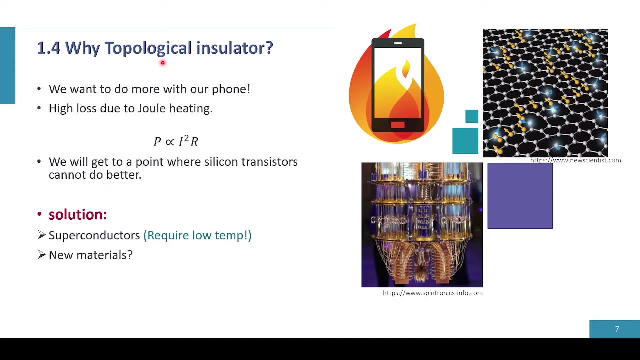 and he connected it with topology and half of the price was actually for that particular thing. now why we need a topological oscillator. the first and important thing is that we want to do more with our phone. yes, we know there are high lows when the electroelectrical 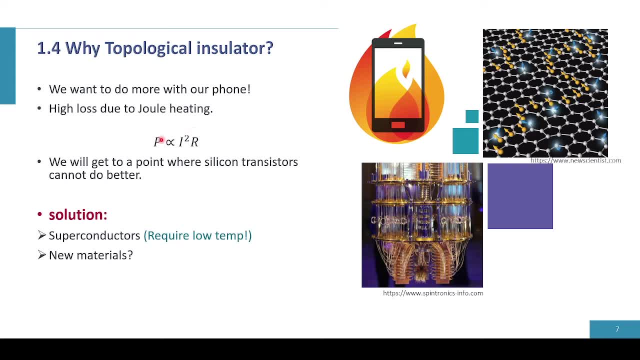 electricity passes through a conductor, the joule city and the most low states that the transistor won't be doing much good in the future and we need some solution, and one solution is indeed the superconductors, but, as we know, it requires a low temperature, even though the high temperature superconductors are. 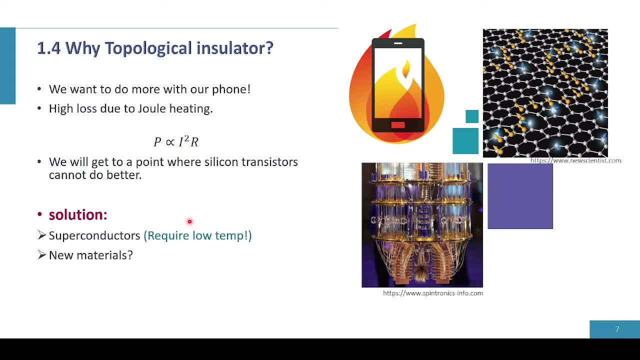 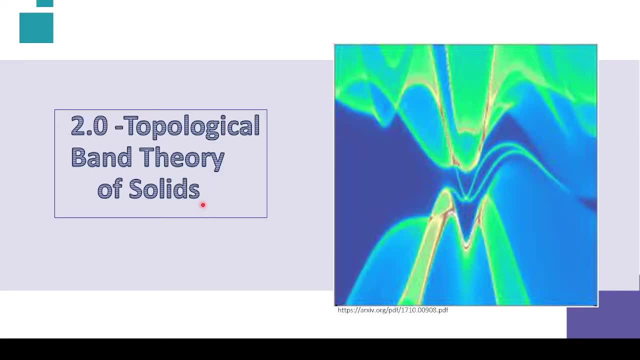 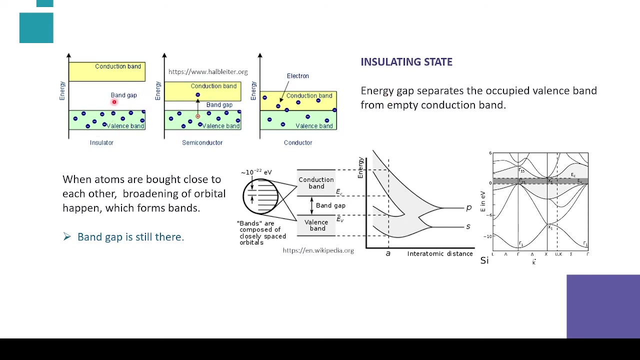 on its way. it's quite challenging, so we need some different new material. so to understand that, let me introduce you to this topological band theory of solid. so to rough refresh, you are understanding. so you know the insulators and semiconductors and the conductors are just having different. 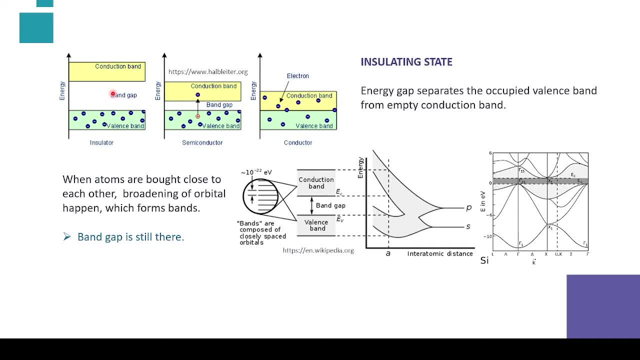 valence. and conduction band: sorry, different band gap so insulators have a having different balance and conduction band- sorry, different band gaps, so insulators have having different band caps. so insulators have having have a big band gap while the conductors have no bank gap, so this band gap differentiated. 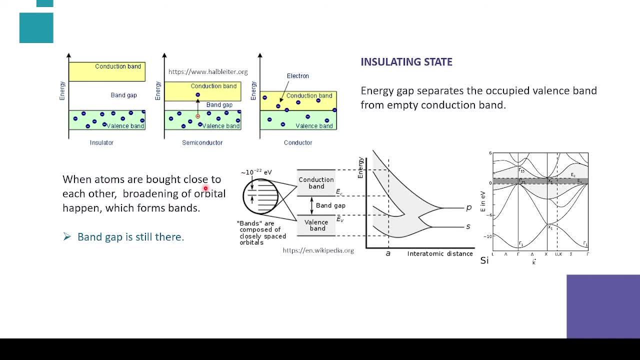 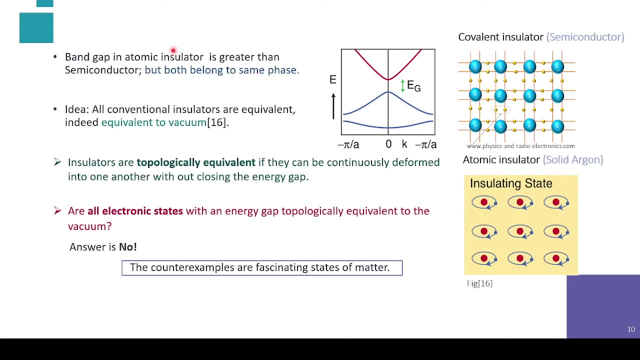 so, when the atoms come close together, uh, they can form orbital overlapping and they form banks, and this is how the band structure formation happen. and this is a simple uh band structure of silicon. now, uh, we say that this is an atomic insulator and this is a covalent insulator, a semiconductor. 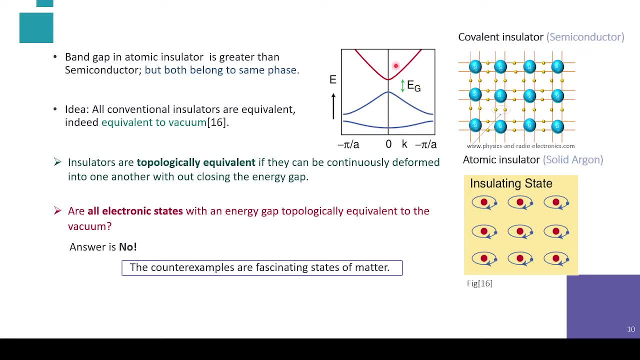 so we know that both of them are actually having a band gap. while the atomic insulator have a wide band gap, the other semiconductor has a small gander, but anyway, both of them have banking. so according to topology we can change. we can slowly change their band gap. 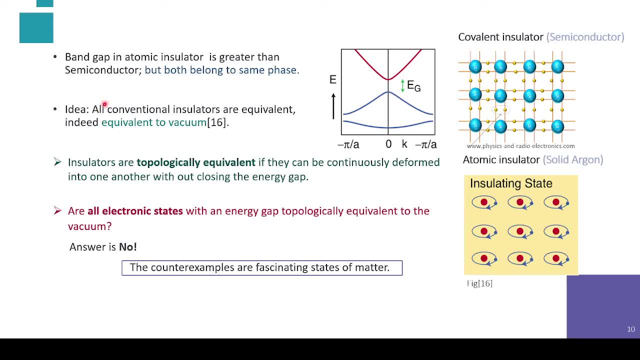 but it should not cross. and another idea is that, uh, this old conventional insulators are actually indeed equivalent to parecer, and they all belongs to the same phase. this is what topology says. so from now on, we only focus on the insulator. so this means that i can slowly deform the band gap. 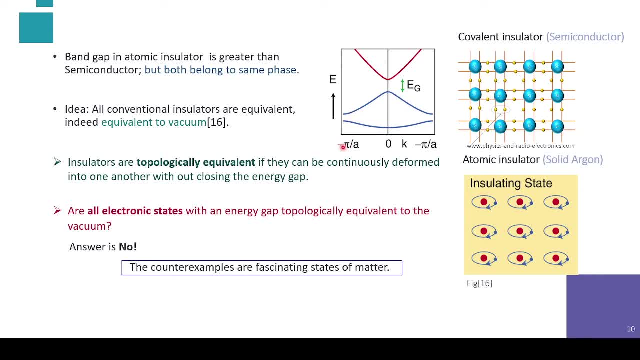 without removing the insulating property. right now, the question is: are all the electronic states, uh, with an energy gap topologically equivalent to the atom, Wes vist? and the answer is actually not. and the yes night, ayutthaya. and next time, are it over the electronic states, uh, with an energy cap topologically equivalent to that of wakewood? and the answer is actually no. and the further of this, that lo to world. it's basically not the problem. but uh, we got aЯ technology in material thing. oh, it should be Eli Nam for it. there's values. what really next riddle which we need to solve are certain more reason of energy. Yes, so from this, all along Bromley, what is effective to do? yes, Ge looks like. 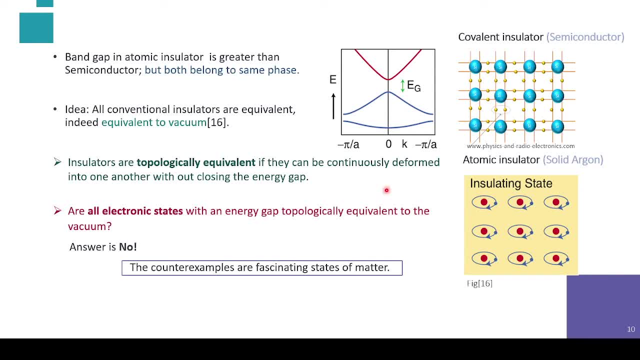 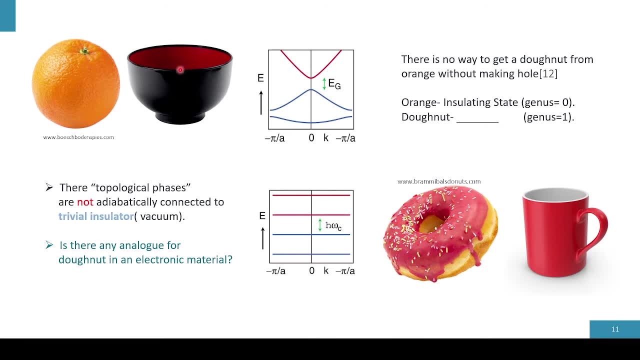 examples will be leading to the fascinating matters that we need, matter that we need. as I told, the orange and a and a bound belongs to the same topological class, they belong to the same face and I will define that by this diagram here. and I say that this is actually an insulating state and I call 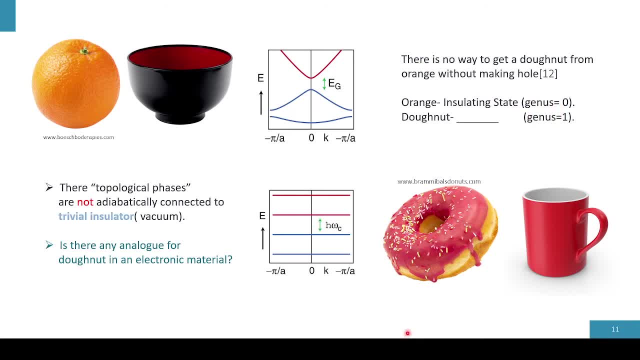 that genus is equal to 0. and here the second phase: this donut and the coffee cup belongs to the same face, and I say that this scanner is equal to 1, but what is that state? I don't know. so my question is: is there any electronic? 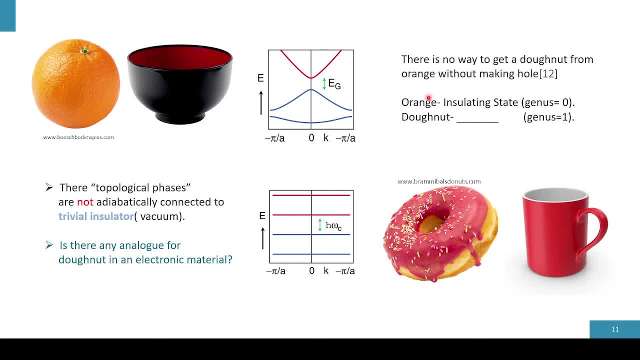 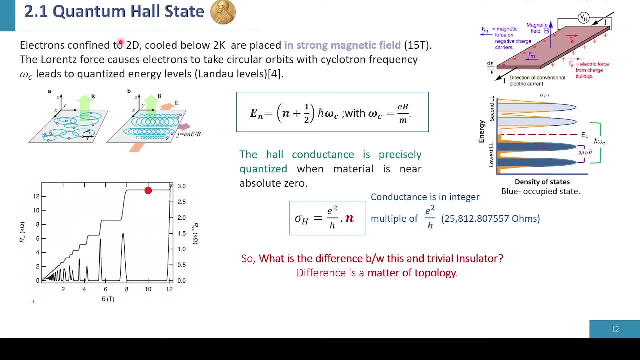 states of matter, electronic state that belongs to this character and that is what I need to find. so as you go hoist here, so as you go hoist here, explain in the quantum Hall effect. explain the quantum Hall effect in Hall effect in detail. in today morning I'll just briefly refurbish, refresh it. so 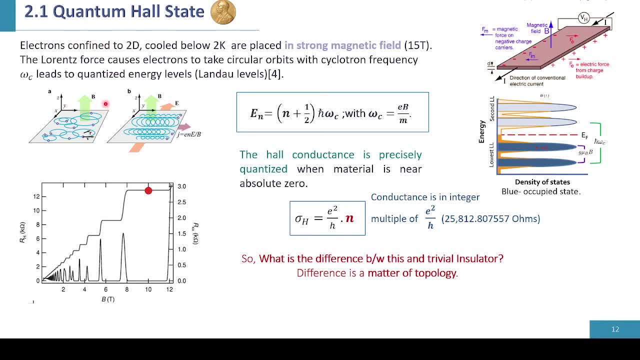 basically the 2d electron gas are confirmed in a matter like this, and you know, it is cooled below in very low temperature and a strong magnetic field- most important strong magnetic field- is applied. so Lawrence force created this anificator, which is there in the number as well. the third difference between the two is the sputtering of the circuit inside the particle which the sputtering of the energy is not enough. so it is not enough and it is not enough, and it is not enough and it is a lot of, it is a lot of data data inside the particle. the second decision about the 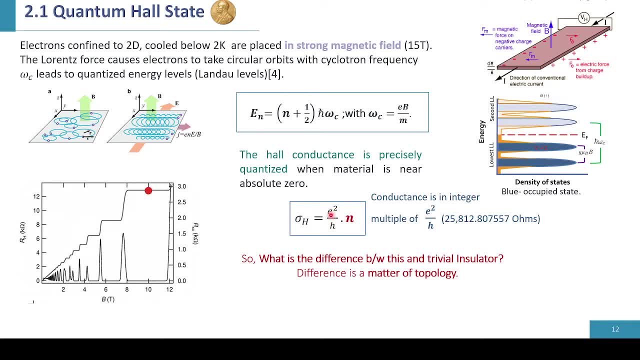 count is to find the quantized long die levels and the contest levels are given by the energy is given by b, NEC plus half edge cross, omega C and the basic idea multiples of E squared by n, that is. keep that in mind. next question is why it is. 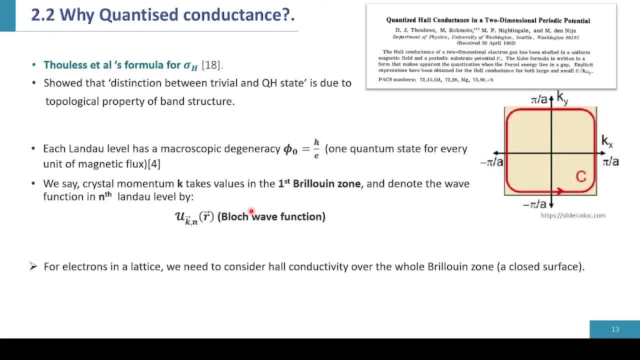 quantized. we need to understand why this quantization is there. so in 1982, professor told us actually derived a formula that connects the quantized hard contact-ends to something called churn number. that means they. he connected this with topology. that's see how did he do it. so this is the 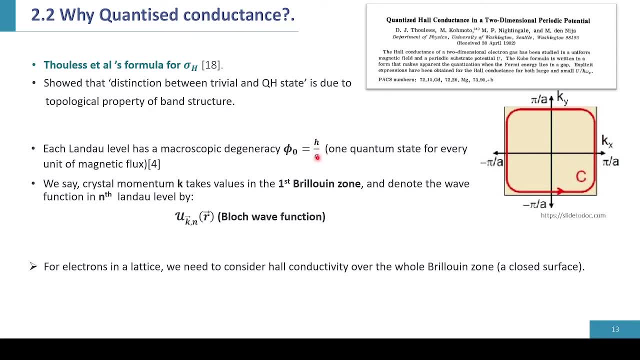 regionality of a land, Medical level: h, h by e. now he defined a wave function, u of K, n, that's a blocked wave function for the nth land available with crystal momentum k in the first below itself. so for electron in the whole light is we need to consider the Hall conductivity over the 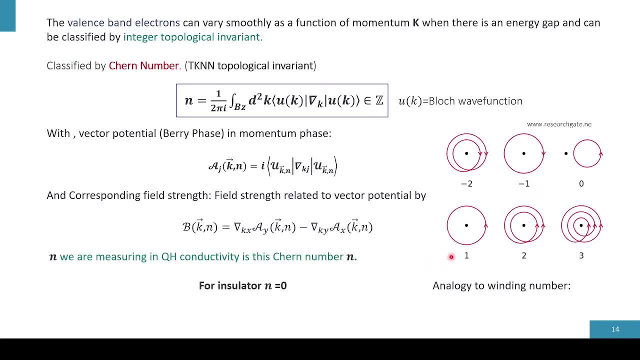 whole Brillouin zone that is a closed surface. now the basically here the valence band electron can actually vary very smoothly as a function of moment fk in the presence of a band gap, energy gap and this can be classified as integer topological invariant. so he found a topological invariant, N, which is defined: 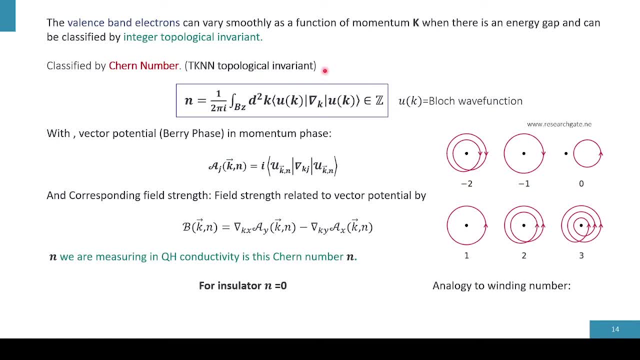 as this one. it is called TKNN, topological invariant, where T stands for the people who were in that paper, and this is also called the Chern number, and this is a function of our vector potential. this thing here in the brackets are defined as is the vector potential of the very place in the moment of space, moment of. 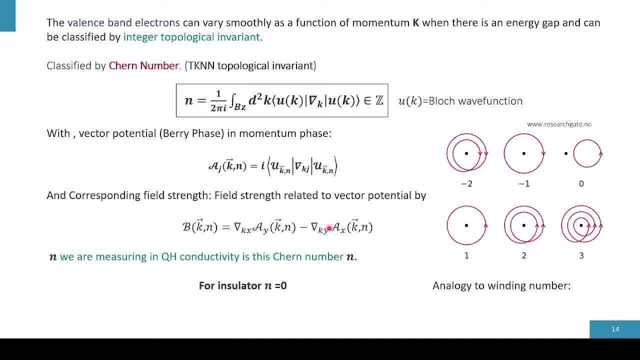 space and the corresponding field sign is given by this. so the basic idea here is that this can be analogous to something called winding number, let's say a system which takes one turn around a point then we call the winding number to be is equal to one if it takes two. 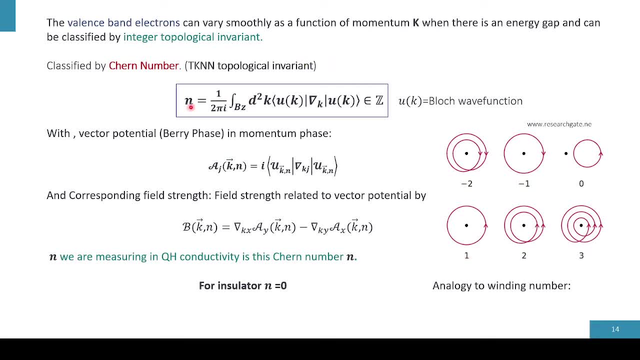 turns, then winding number is equal to, and so so here, this N is actually the N which I told you, to keep it in mind, the integer quantum, that, that integer, that is this. so he, thereby he connected the quantization of the Hall effect into this topological invariant N. this is the function and this N actually tells about. 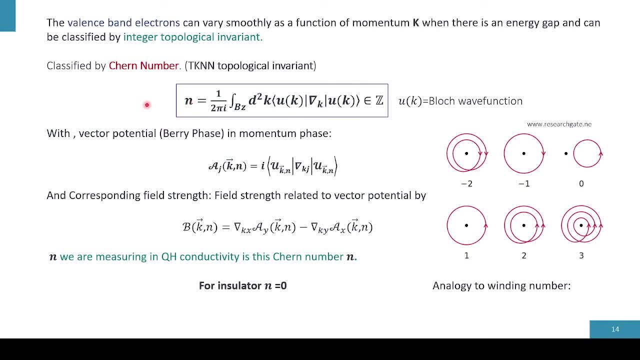 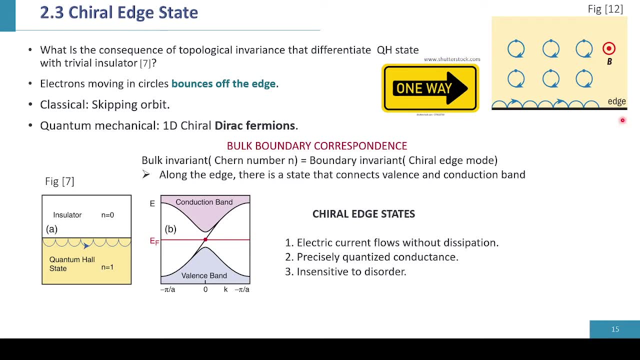 the edge mode that carries the current. we will learn about that in a minute. so let's see what the edge state is. in the normal presence of the magnetic field, the electron will take a circular turn, as I shown here, but you know what happens. so what happens at the edge state? in the edge state they actually bounces off like 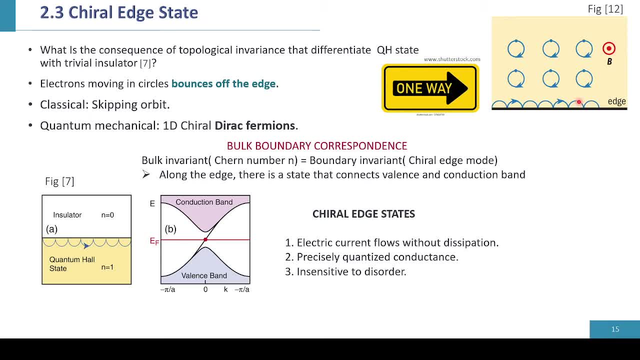 this and classically we can say this as the skipping orbit in quantum mechanics we call it one-dimensional spiral distance Gerber R � is equal to championship R Freud is equal to a gate where this is we will need to apply these two Bali in order to apply some 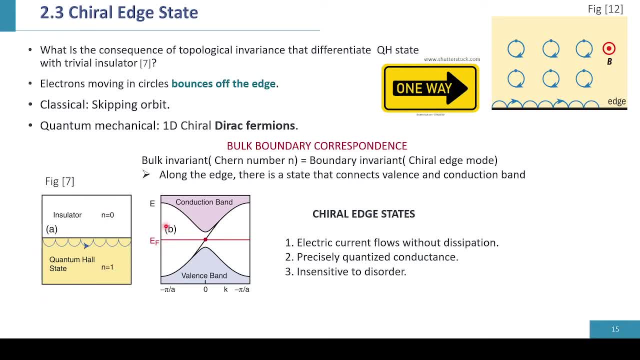 for one Wi-Fi. so theравля in quantum mechanics, r bar is equal to fear and an interior chains is of course identified in quantum mechanics. the churn number actually connects the bulk part, bulk invariant here and also related to the boundary invariant which is given by the chiral edge mode, and this is the usual conduction and 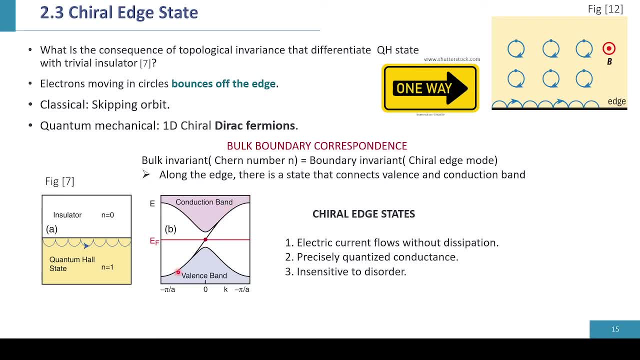 valence band and you can see here, there is a small edge state here and the valence and the conduction band has a energy gap and they don't do anything. they are insulators, but this edge state is there and that is special. and what are the properties of this chiral edge state? the electric current flow. 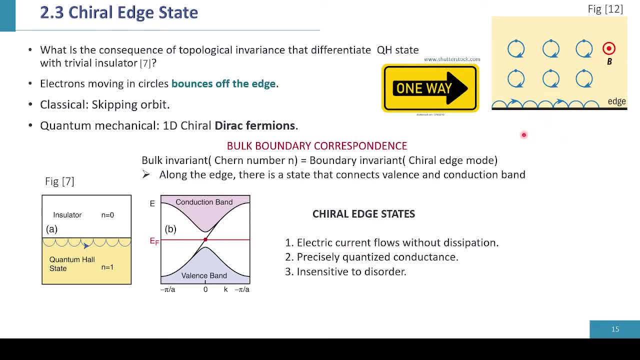 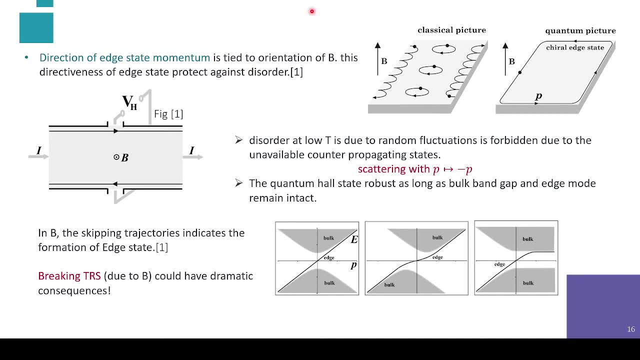 without dissipation and they are precisely quantized and they are insensitive to this order. now let's look at this edge mode in detail. so this is the classical picture for skipping over and this is the quantum picture where the chiral edge state is there, and special is this momentum. 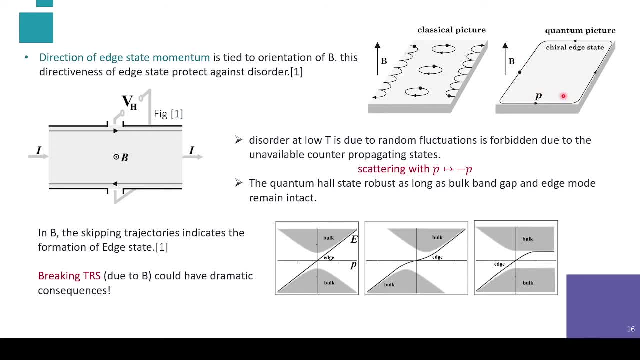 and the spin are actually locked. it is the momentum. spin locking is there. we will explain it later in plus few slides. so here you know. at dot m raised also, there are many random fluctuations, but since the counter propagating state is not there, there is no scattering. that is this state. 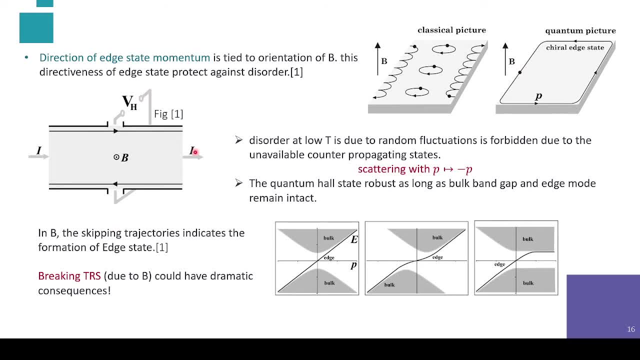 is actually very robust and this is how the usual connection look like. you have the uh high voltage measured here. this is the conventional current flowing the magnetic field is played for, particular this one. this is how it looks like. you can see the state here and you have to understand the time reversal symmetry in the presence of magnetic field, actually the 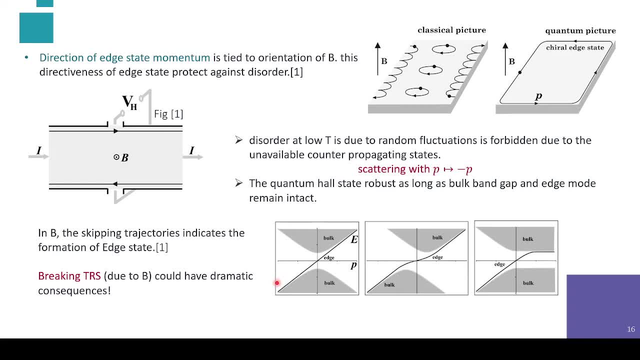 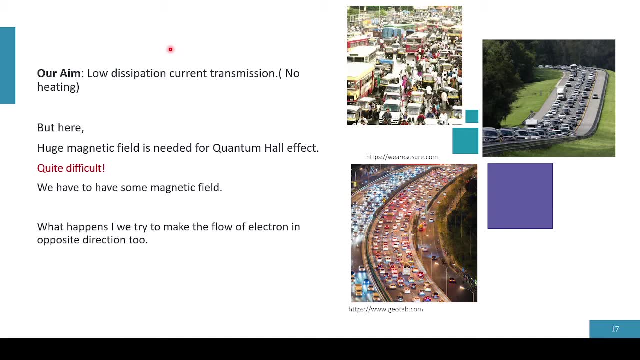 time, reversal symmetry is breaking, and this has a dramatic consequence that i'll explain in few slides. so what is our aim? our aim is actually to get a low dissipative current transmission. that is, uh, there should be no heating at all, but uh, as i told, a huge magnetic field is needed. 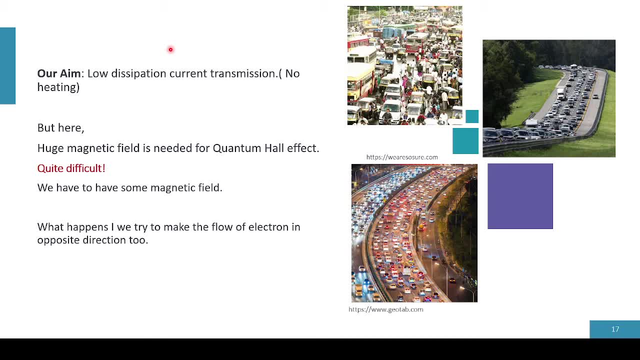 but that is not possible. we can't carry the magnetic, huge magnetic field in our with us with no phone right, so it is quite difficult. so we need to get a magnet within the material. that is what we need. we need a magnetic field within the material, and this is how this picture depicts how the usual conductor looks like and this: 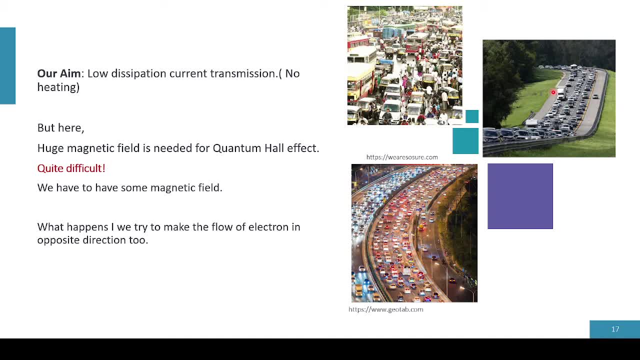 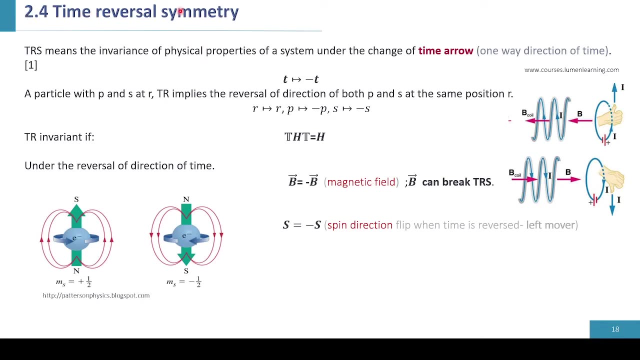 is the you know that i was mentioning, and this is how what we need. we need to allow the electron to flow in opposite direction and then see: will we get? it will permit or not. so before continuing, let me explain what the time reversal symmetry is. so time reversal symmetry just means that the property of the system should be unchanged. 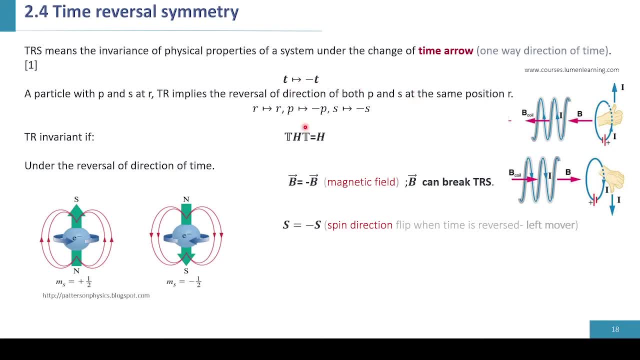 when the time is reversed. so if a hamiltonian is there and time reversal operator is update, then hamiltonian will should be just the same. but a current is flowing, like this, in one direction. that is so when we reverse the current flow, that is the time reverse the operator is applied. 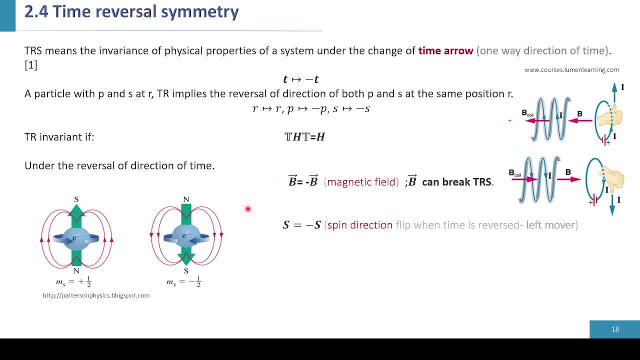 what you can see here, that the magnetic field direction is changed. so the magnetic field direction will change when time reversal thing happen. so basically the conclusion is that magnetic field actually can break the time covers. Oh, so you can see the electronic before in one direction and liquid will be in a down direction. 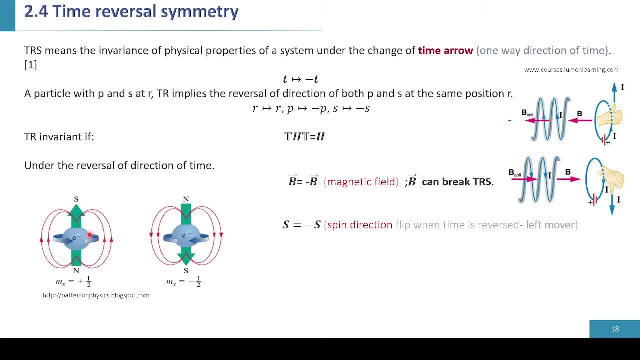 and if the electron flows in the upper direction, other direction spins in the other direction, magnetic field in the opposite direction. so spin also get flipped when the time is reversed or the left mover become the like left right mover. now one more theory to understand is the crammer's theorem. this just 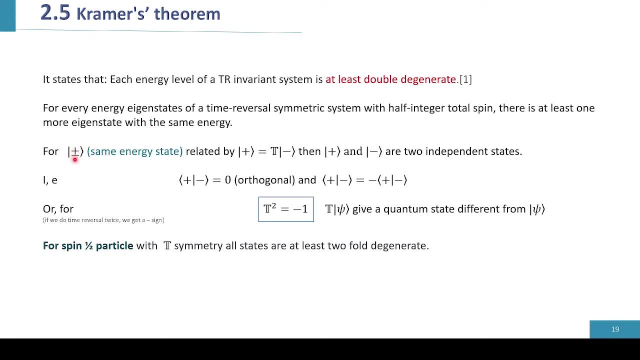 states that uh, if we have a state uh which is in the behavior state, this plus or minus, which is in the same energy state and is related by this time reversal operator, then this system should have two independent states. that just means that for a spin half particle uh which obeys the time reversal symmetry, then all the state has to be two-fold: uh, degenerate. 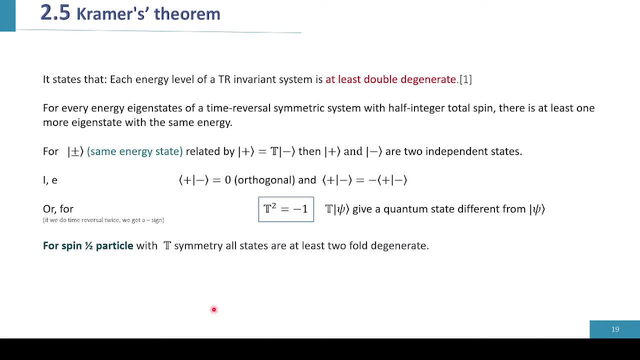 that means if one uh up spin is there, then other down spin has to be there in a same energy state. that's the basic idea. so if you apply the time reversal symmetry twice, then you have to get a minus one. that means the uh other state has to be different. 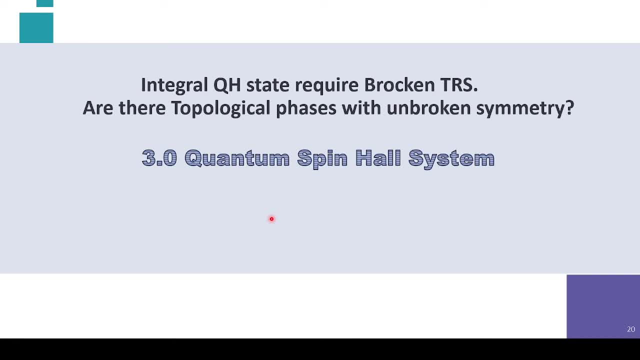 from the first one. so, uh. so, as i told, the integer integral quantum halt state requires a broken symmetry and we need a magnetic field inside. that means we don't need a- uh, a broken symmetry. so is there any topological basis with this unbroken symmetry that we need? 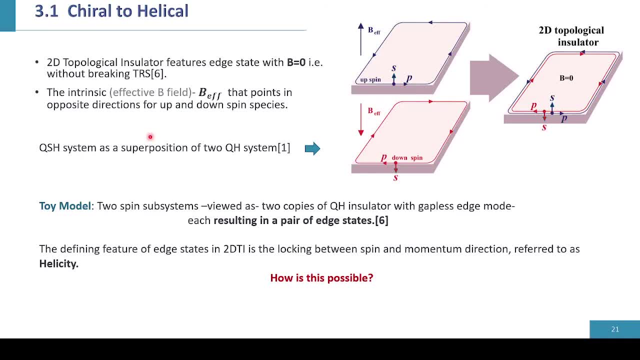 to find. so i'll propose one toy model. toy model like this, that is uh. when electron flows along the edge state we know a magnetic field will be produced. similarly, if the electron flows in the opposite direction, the magnetic field will be in other direction. so if i combine both, 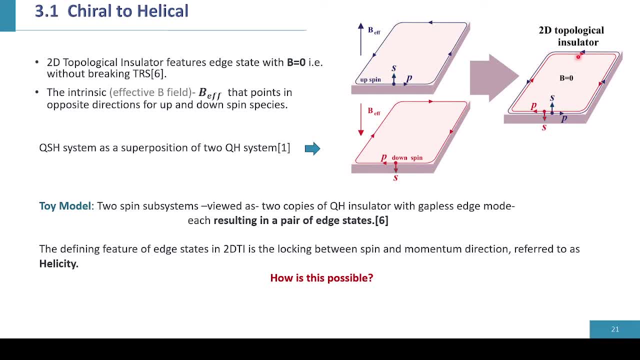 i'll get a state like this and i call this topological 2d, topological insulator. this is what we need. here we have a inbuilt magnetic field that means the external magnetic field is zero. so here the quantum spin heart system, uh, has a super position of two quantum heart system. so i call this is. 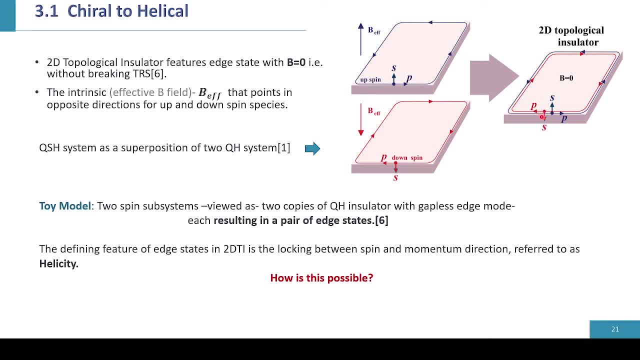 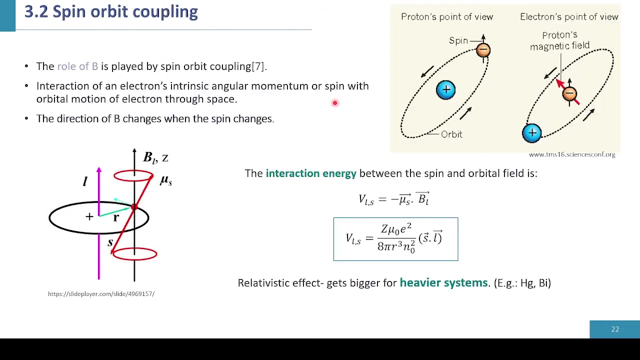 actually called the quantum spin heart system, and this is a toy model with the commerce theorem. uh, we get, uh, a pair of a state like this. and you know, here also the spin and momentum is low. and how is this possible? how can this be done? how is it done? the answer is very simple. it is because of this spin orbit coupling. 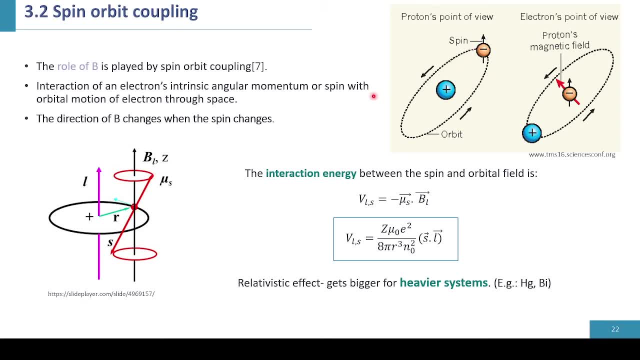 you know, spin, uh, electron has its own speed and it revolves around the nucleus and that causes a magnetic moment for the orbit and for the spin. so we have a magnetic moment for spin and this nucleus here. so the interaction energy is actually related with the both of them. 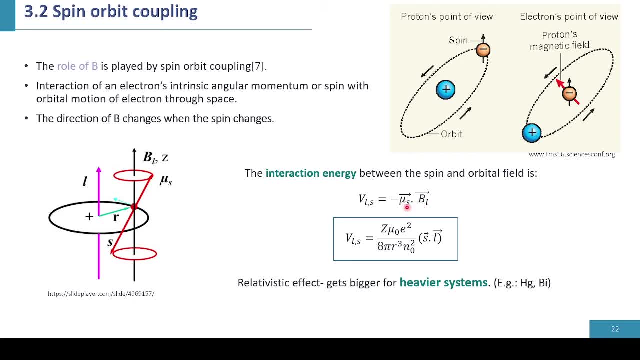 angulo angular momentum of the speed and angular momentum of the order. and also you can see one important fact: that the interaction energy here is actually related directly. proportion to z, that is the atomic number. that means for heavier system we'll be having high spin orbit, coupling heavier 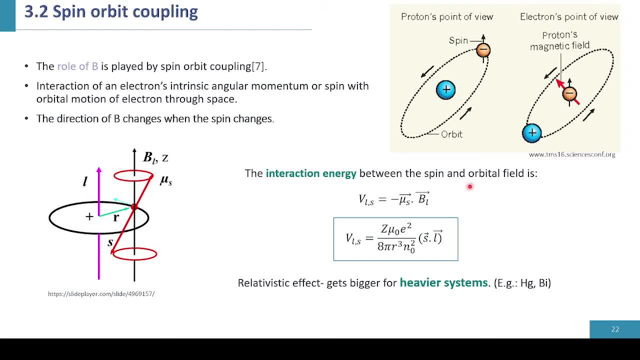 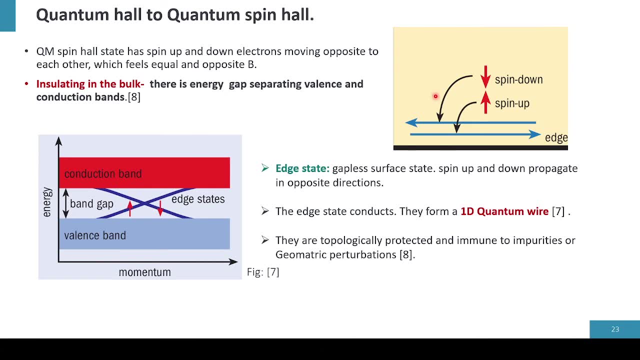 system is mercury with, that's all. so this is very important here. so just to summarize the quantum spin heart system. so this is very important here. so just to summarize the quantum spin heart system. so just to summarize the quantum spin heart system, As I told here, the quantum spin hard state has the conduction band and balance band and 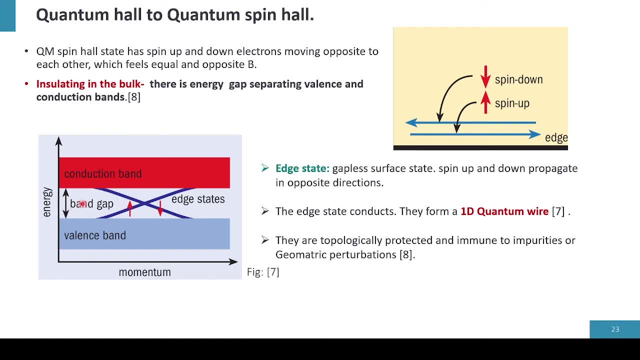 it is separated by a band gap and the system is insulating. but we have edge state. we have two edge state here, with each one corresponding to opposite spin, like this, and this is nothing but similar to that of the one-dimensional quantum wire: The edge state is what is conducting, but the other thing, the conduction and balance band. 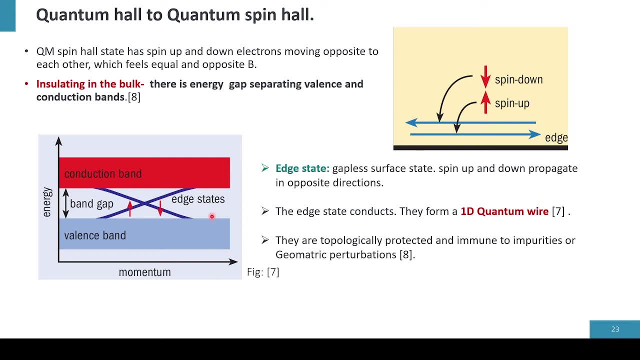 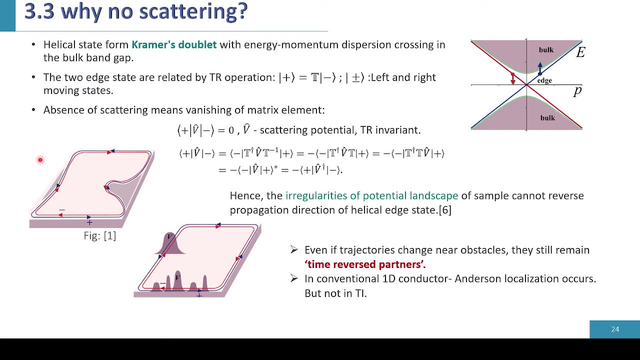 has energy gap and that whole system is actually insulating and this is actually also immune to impurities of other perturbations. and why there is why it is immune, why there is no scattering or so on. the explanation is very simple here. this is the picture, you know. 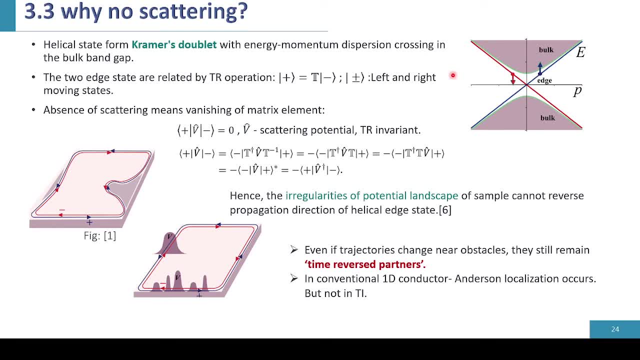 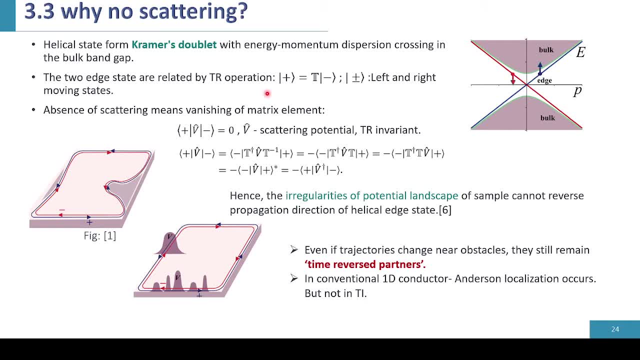 So absence of scattering means that the vector, the scattering potential, the metric element of the scattering potential will become zero. So if I apply so, consider a, consider a potential V, and we apply the Kramer's theorem And time reversal operator, and you see that this metric element becomes zero. that is, 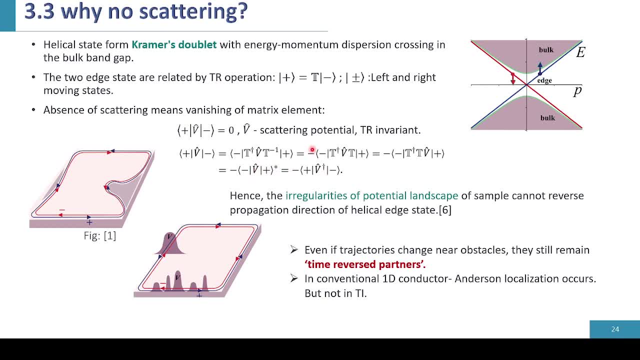 the V is equal to V dagger, That means the metric element is zero, that means there is no scattering at all. So you can see here, even though some irregularities in this potential region, here comes into play, this, just this trajectory of the motion of- sorry, the trajectory of our spin system, edge. 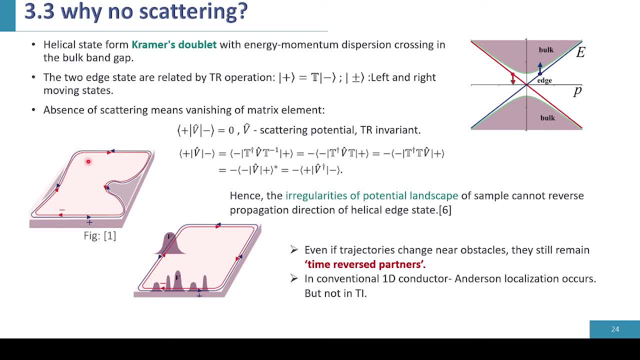 state is just flowing. Let me show you: the city is not at all scattered or it stays the same. That means they stay as a time reversed partner, As Nirdian Thomas Alex explained in the Anderson localization for the one-dimensional conductor. but here, even though this conductor can be called as a one-dimensional head state, 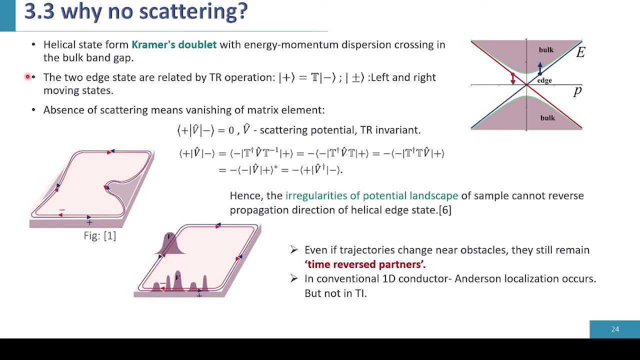 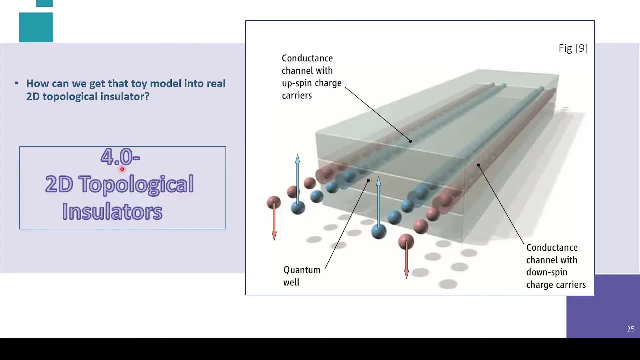 this does not have any Anderson localization. that won't happen in this topological insulator. Now, I was explaining you about the toy model, right? So now let's go into the actual discovery. This is just a simple cartoon explaining what I told you to a state like this here. Okay, 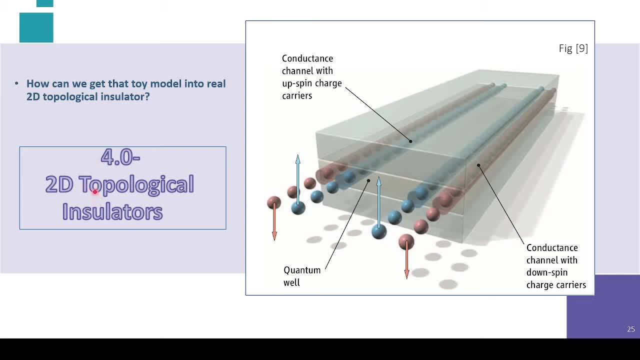 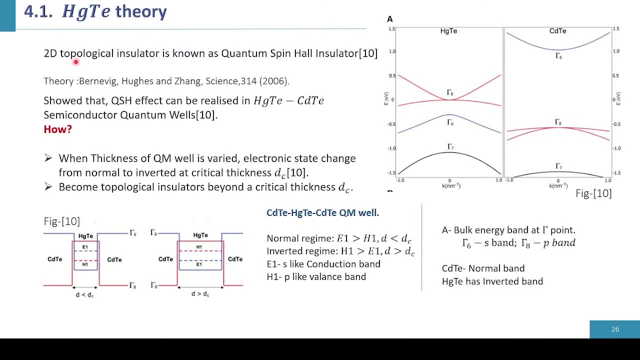 so now I'm going to this topological insulator. You know, so you know the quantum spin heart state. the quantum spin heart insulator is actually what is called the 2D topological insulator that you have to keep in mind. Okay, so I was actually explaining. 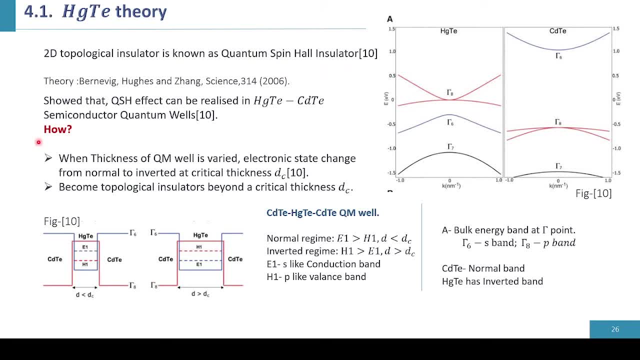 to you about the 2D topological insulator. So in 2006, Birnbeck, Huggins and Pang gave a theoretical prediction. They said: well, if you make a 2D topological Insulator, then the O6-g mercury telluride could. 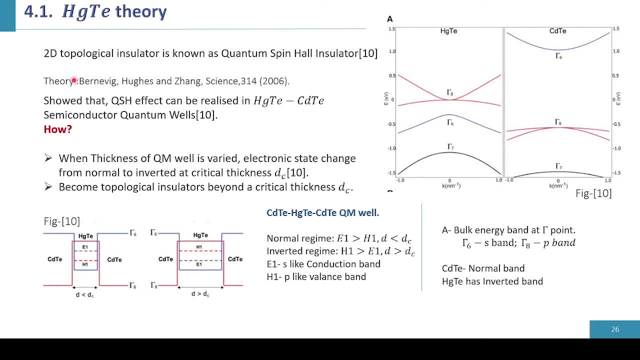 be a best candidate for the top 2D topological insulator. This is just the theory. So what they did is they told that if you make a quantum bell out of mercury telluride and cadmium telluride, then this should be topological insulator. So you can see, this is the band structure. 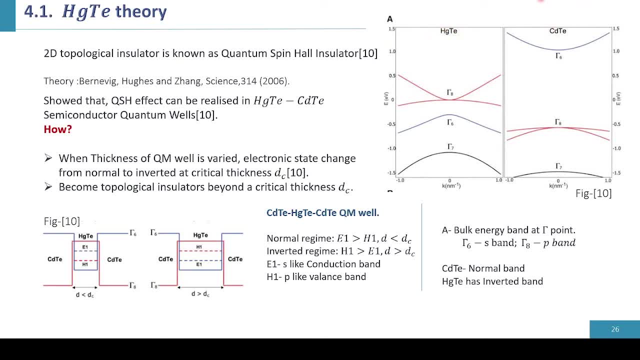 of mercury telluride and this is the band structure of cadmium telluride. And if I say the red line correspond to the valence band and the blue line correspond to the valence band, then you can use the valence band. It will be a chocolate ball And you can add this little bit of the chocolate ball. 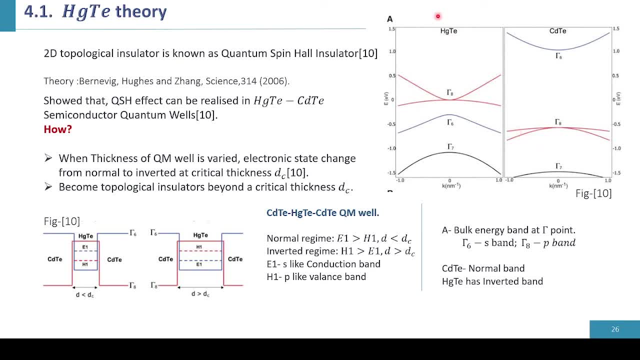 blue one does not be the conduction band. you can see a peculiarity in mercury tiller that is here the valence band is actually above the conduction band. that should not be the case here. this is the normal conduction band is above the valence band. why this is so? keep that in mind, okay. so, uh, this. 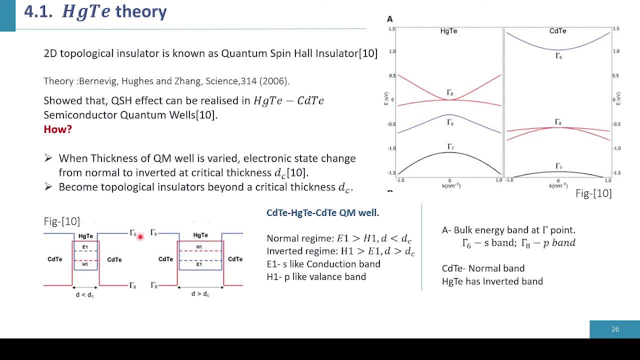 is the quantum well. this is how the quantum well structure looks like. so e1 is the conduction band and the h1 is the valence band. so this has a thickness d. they say that if the thickness d is less than something a critical thickness, then this has a normal normal. 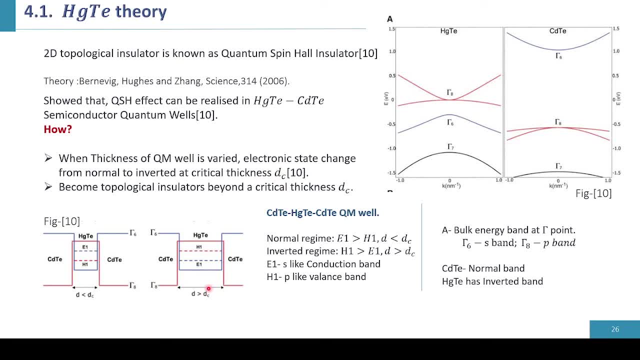 band structure. but when the thickness d becomes greater than the critical thickness dc, then this becomes topological insulators. that means the band inversion will be happening. so the main idea is that for a band, for a topological insulator to form a band, inversion has to be taken. it has to take this: 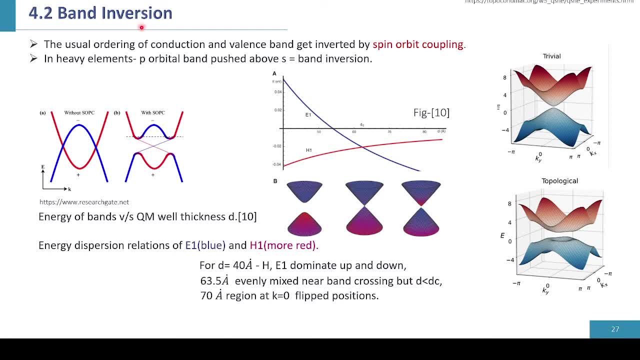 now let me explain about the band inversion in detail. what is the reason for that question? simple, as i said. as i told, it is nothing but the p-orbit coupling. so in heavier metals, uh, the p-orbital band actually is pushed above the s band and band inversion will be happening. so this is how the band. 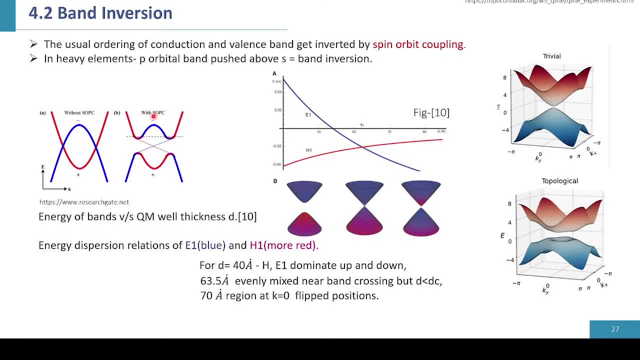 without spin orbit coupling look like. and this is how the bands with spin orbit coupling looks like. so this is a energy of a band versus the quantum. well, thickness d you can see here e1, uh, e1 is this conduction band and the h1 here is the one red one is the valence band. 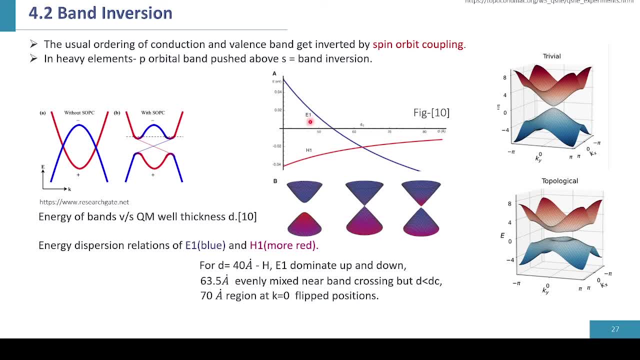 and in the normal case for d is equal to 40 ampstrom. you can see the valence conduction band is above the valence band, but when the thickness becomes 63.5 ampstrom it is becoming strong. so the band is crossing actually, but still it is not above because it. 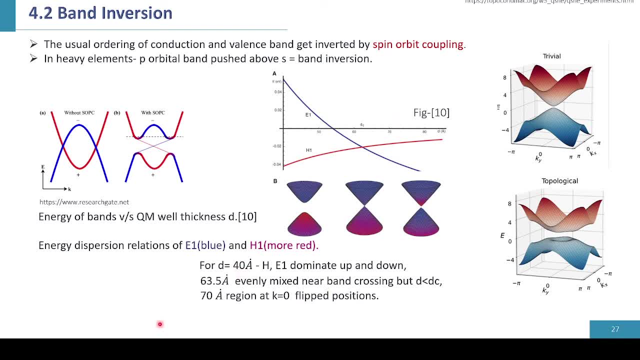 is less than dc, but for d greater than dc you can see at around 70 ampstrom at the k point the bandant version is happening. but this is how the band- a normal band in 3d and inverted band in 3d- looks like. 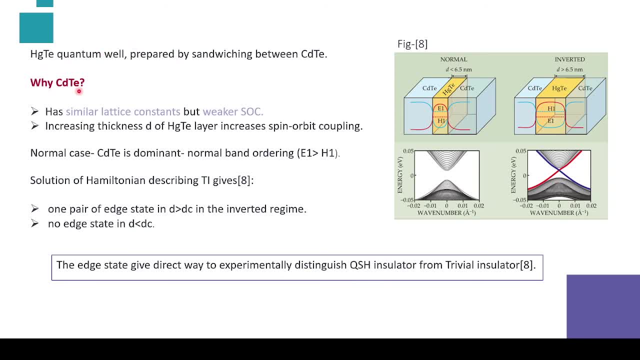 now okay. next question is: why did we use the cadmium right along with the mercury delay? because it has a similar lattice constant. both of them have similar lattice concerns, so you can get the k point diverse due to� easily compare them. Also, second thing is that Gantt-Mittell rate has a weaker spin-orbit coupling. 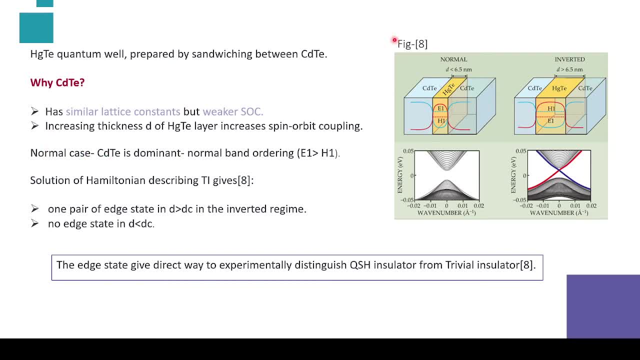 Now, in the normal case the Gantt-Mittell rate dominates. that is the normal band ordering should happen. but in the inverted case, that is, after spin-orbit couplings come into play, the band inversion happens. So if I write it, if you write a Hamiltonian describing this topological 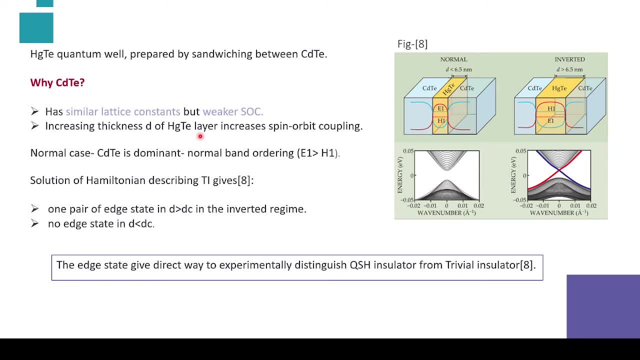 this 2D topological insulator, we get the solution which gives you one pair of x? d for d greater than dc. that is the inverted regime, and you will find no x state for d less than dc. Now, finally, we have came to the idea that I explained in the beginning: The x state. 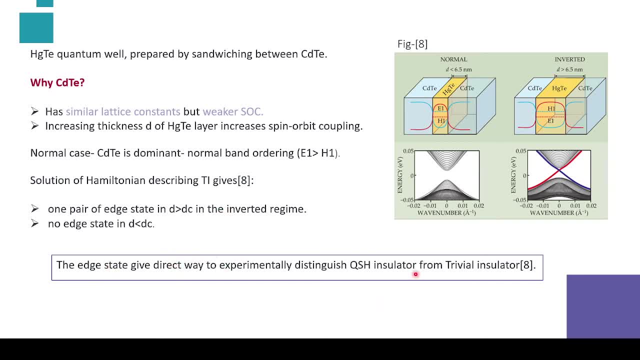 gives the direct way to experimentally distribute the quantum insulator from the trivial insulator, That is, to distinguish between orange and dark. Yeah, So if we can experimentally find this one, then we are done. We can easily say that we have discovered the topological insulator. 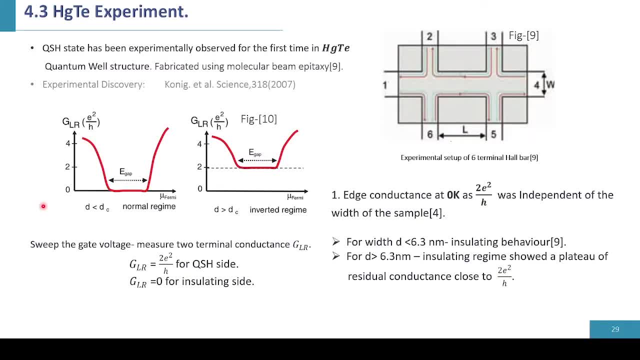 2D topological insulator. So experiment is going As I told in the previous slides. the quantum Hall state, the first one, is experimentally observed in the same theoretical prediction, that is the Mercury-Tel right. The quantum bed structure was actually fabricated by sandwiching HGT and catmintene right. 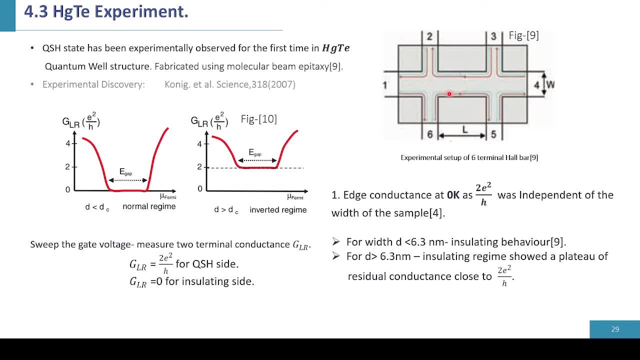 And this is how the experimental setup, the 6-terminal Hall bar, looks like. We have 6-terminal with a length here and the width this one. Now the thickness is actually overlapping. that means you can vary the thickness there. Anyway, for d less than dc, here you can see the Hall 1, 1, 3.. So with x I see the. 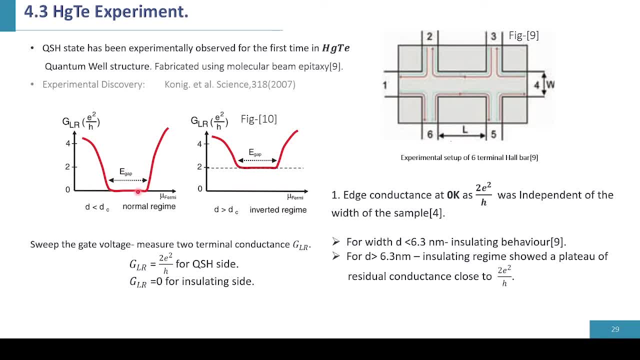 Hall contactance and we vary the gate voltage also. So you can see the Hall contactance is 0 for d less than dc- normal trajectory And for d greater than dc we have the quantized Hall contactance. It is around 2, that means 2d squared by h. 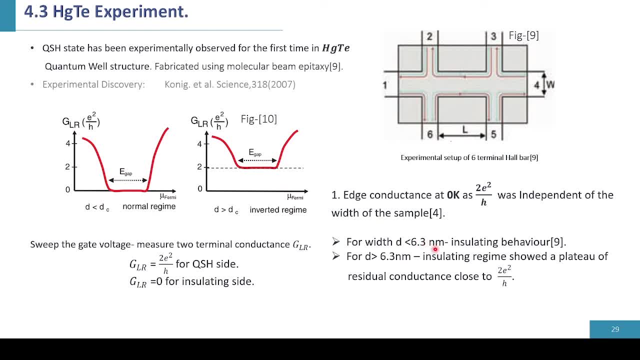 So this is the thickness that I use. for d less than 6.3 nanometer it showed insulating behavior, And for d greater than 6.3 nanometer it showed a conductive material. that means it became a topological insulator, and this is the 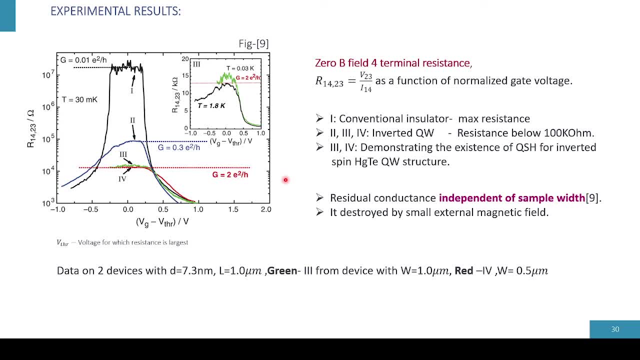 actual experimental result looks like you can see here this. also remember that this is in the zero magnetic field, that we are not applying any external magnetic field. and this one is for the Hall resistance and the voltage applied- gate voltage here. so you can see here for for a normal conventional insulator you can see a maximum resistance. it's. 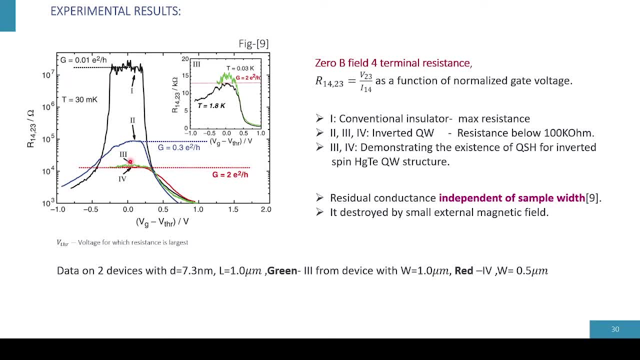 almost more than 10, raise to 7 ohm for this two, three and four. almost this is insulating. the resistance is coming below 100 kilo and especially for three and four, that is the inverter region. you can see the Hall conductor. the resistance has increased drastically. 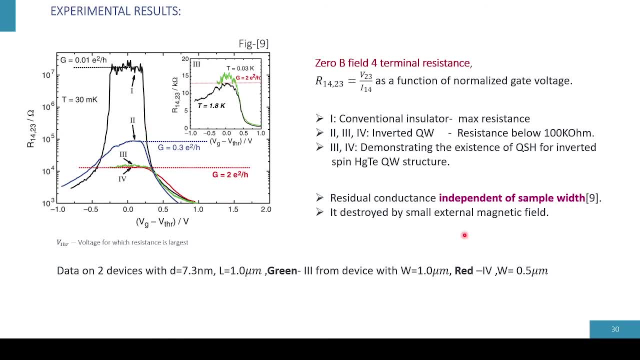 so this is the two important facts are this versus the silver: conductance is actually independent of the width of the sample, the beat I showed you before, and if you apply an external magnitude field then this is distort. that means the project is face is distraught. so the green and the red one, exactly for 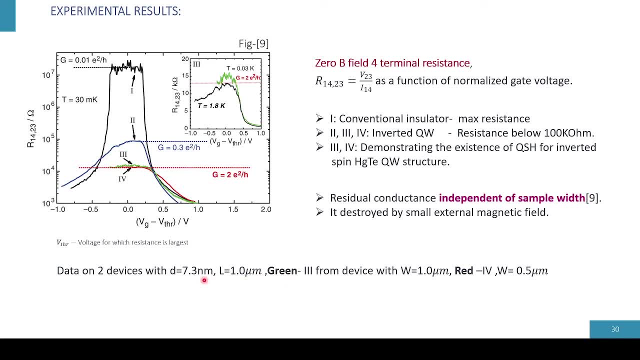 different width, it's for 7.3 nanometer. you can see here which is one micrometer and one. yeah sorry, one micrometer and 0.5 micrometer and anyway, this. this is the result that they got. Now we are heading towards the 3D topological. 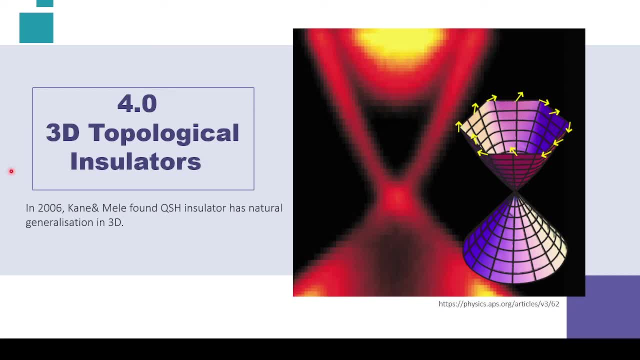 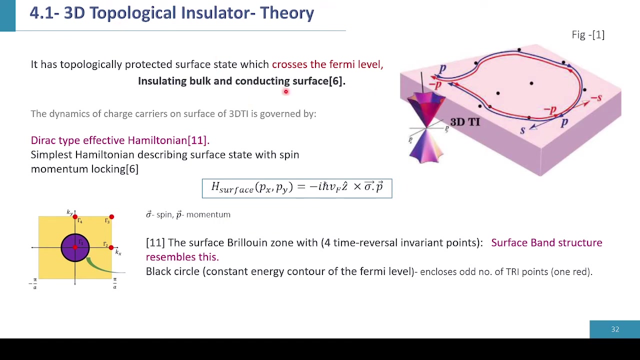 insulator. So in 2006, the theoretical prediction, the theoretical Kane and Millet, actually theoretically predicted the existence of the possibility of the existence of a 3D topological insulator. and you know, in the previous 2D topological insulator we had a insulating surface state and we had a 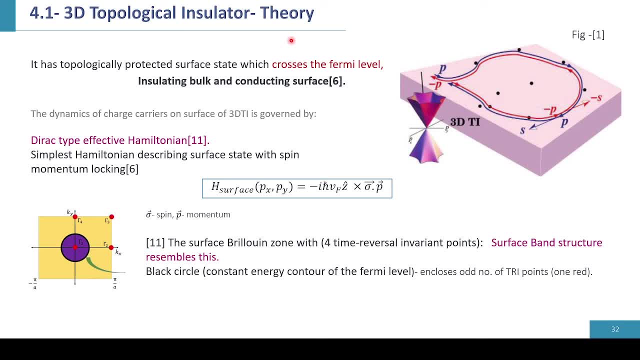 conducting edge state, and here we have a insulating butt state and conducting surface state. That's it. So here the surface state actually crosses the Fermi level, which you can see later. and here, for this theoretical understanding, the simplest Hamiltonian that can describe this 3D topological insulator phase is actually: 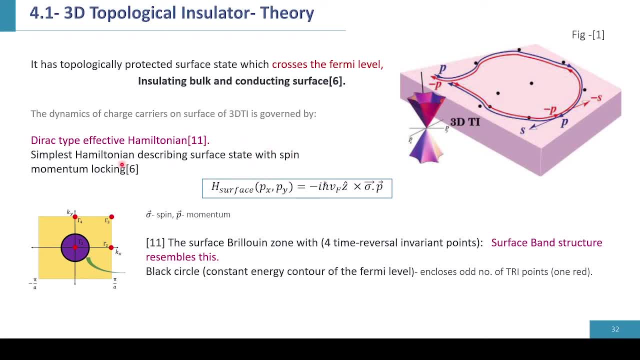 given by this one, where we consider the spin and momentum working as done before. So the Hamiltonian along the xy plane, the momentum along Px and Py is equal to minus Ix, cross, Vf, z diagonal, plus sigma dot p, where sigma is a spin and p is the mountains, and this 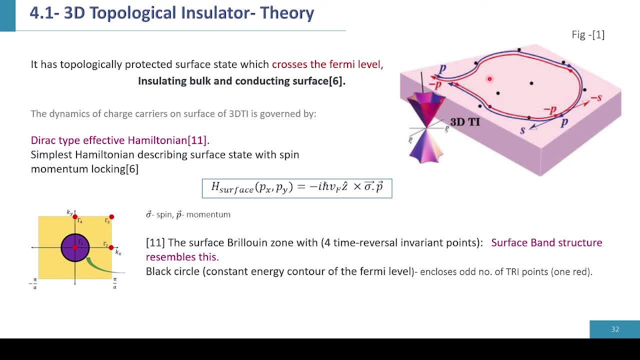 is how the surface state is just a diagram or a carton of surface state. So the surface below it's zone has what time achievable? average 26.6マ worldwide straight, an us 4 time reversal invariants. several edits: this is the surface bank structure. almost looks like this. and then tomorrow 0. 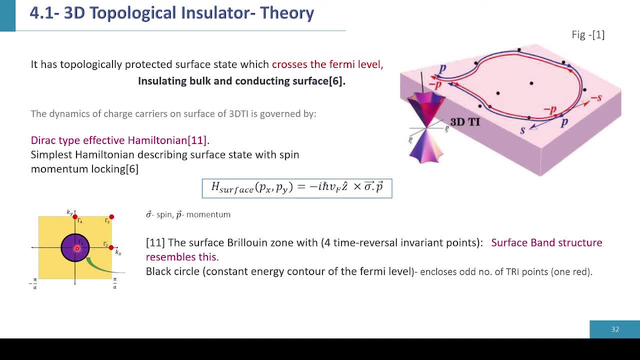 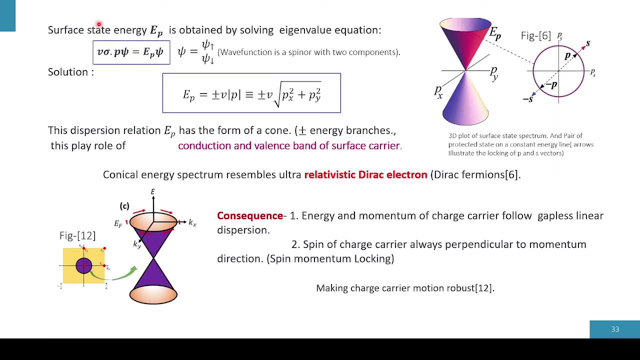 structure almost looks like this and the point at the center, the black point here, is actually the constant energy equal to uh. that's in the first below, first of the fermi level, which maybe you can understand in the further slides. so the surface state energy, ep, can be obtained. 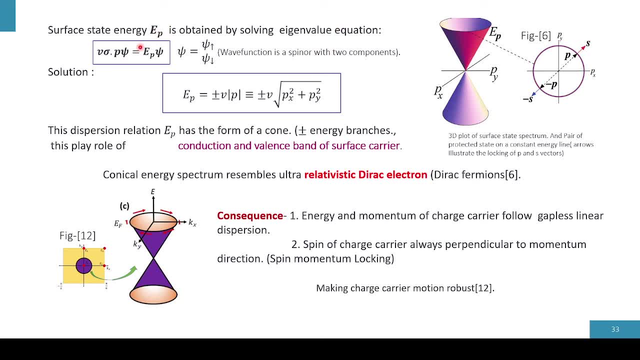 by solving the eigenvalue equation similar to the hydronian. uh told you before, and this is actually b sigma p. psi is equal to energy, state energy, surface state energy into psi, where psi is described by the wave function in the spin on and you can see this gives a solution as this one and 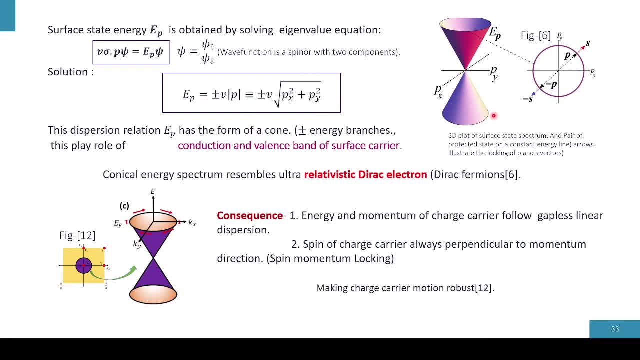 this describes a conical structure with this plus and minus energy branches being the conduction, and values function, and what are the consequences? the consequence that the energy and the momentum of the charge carrier follow a gapless linear dispersion. that's used property shown by a direct electron. 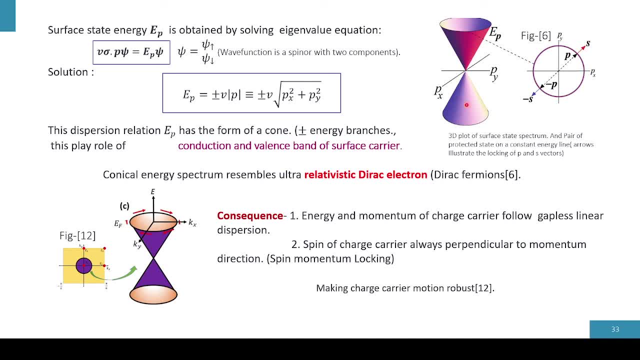 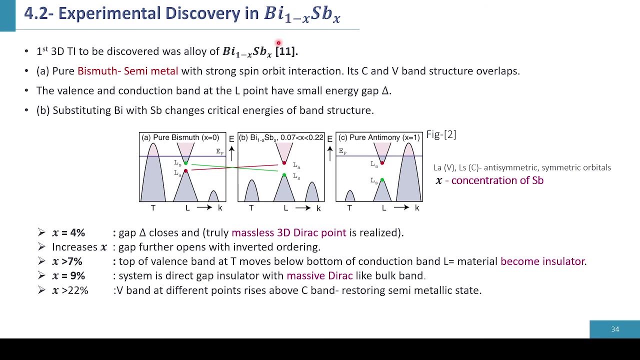 for the direct, direct, relative, sorry, direct formula, right, linear dispersion at the spin. here you can see the spin and momentum are perpendicular. that spin momentum blocking is there again here, uh, making them uh more robust. now we can experimentally discover the uh, this one. so here you can see. 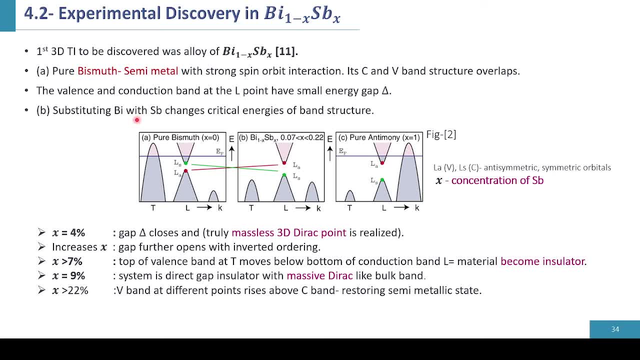 uh, bismuth antimony alloy is induced and this is the band structure for pure, pure, pure bismuth uh, this with. here the valence band stays above the conduction band. here, and you can see, there we were reducing the thickness of the beat, but here we are reducing, we are changing the concentration. 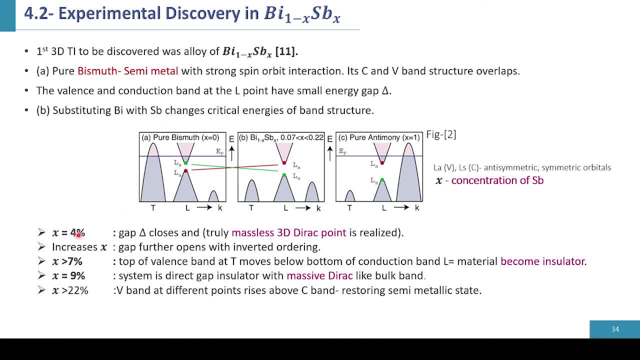 of sp. so for a concentration of sp four percent, you can see the fan crossing happens here. that means the master's beauty direct point is realized at this point. but when you increase the concentration and you close, uh, greater than nine percent, or greater than seven percent, this is moving down. 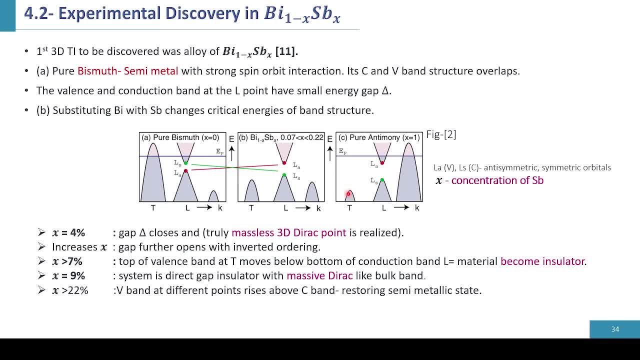 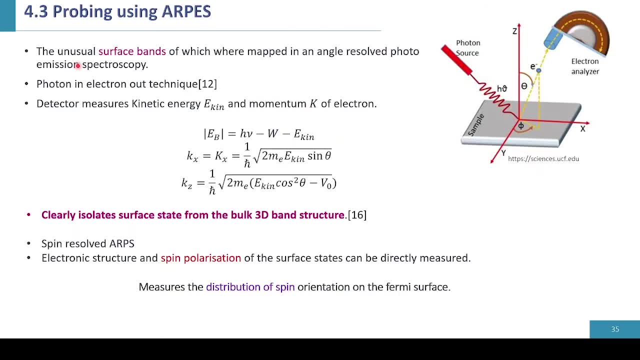 and now this is becoming an oscillator and if you increase it further then it becomes the usual semi metal. okay, which shows the semi metal behavior. i hope you how you can probe it extremely. the probing is done using a plus method, airps method, the simple one, right, you all know the electron in the photon in and 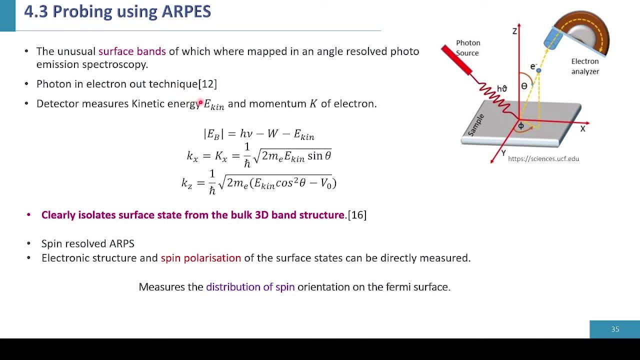 electron out, so you can measure the change in the kinetic energy and the moment and you can get the details about this. and this thing is related by related to the angle and the potential. anyway, we can clearly isolate the, the bulk state, from the surface state using a purpose method and 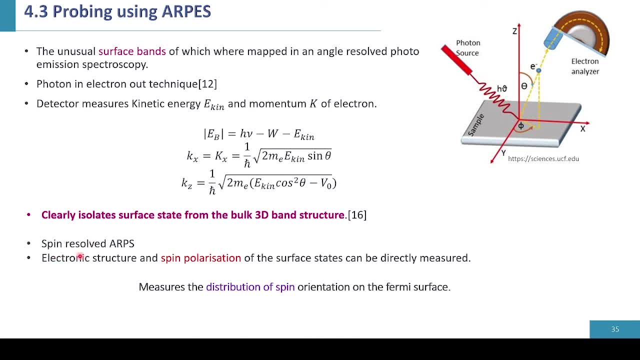 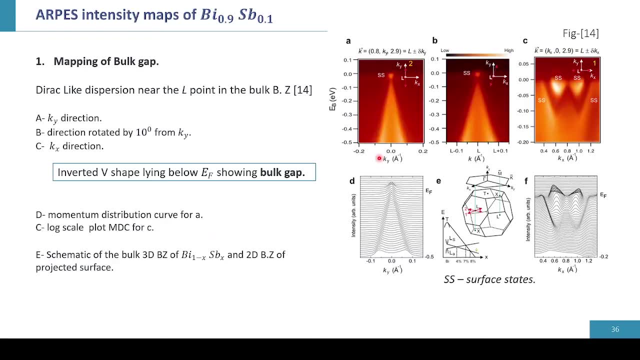 a much detailed review, detailed experiment method is still to solve one where you can actually get the screen distribution on the surface, the fermi surface, using this method. so this is the arps intensity map and here what they did. is they actually the intensity map of the case space? they actually cut through the l points. 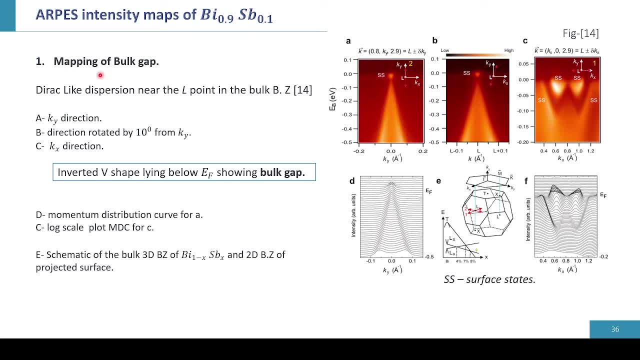 here of the bulk 3d glovin zone. this is actually the third below in zone anyway, this is the main is the cut along the ky direction. this is around the ky direction, tilted by 10 degree angle, and this is along the kx test. anyway, you can see that, uh, this inverted fan shape is lying below the 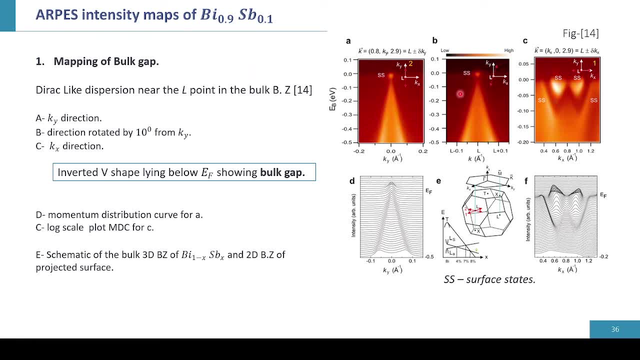 fermi surface. this is, you know, the surfacing, so it blows. it is lying below the fermi surface. that means this has a small band gap somewhere here. that means this is the bulk gap. so this material is actually showing the bulk gap. so these are just the moment of distribution curves. 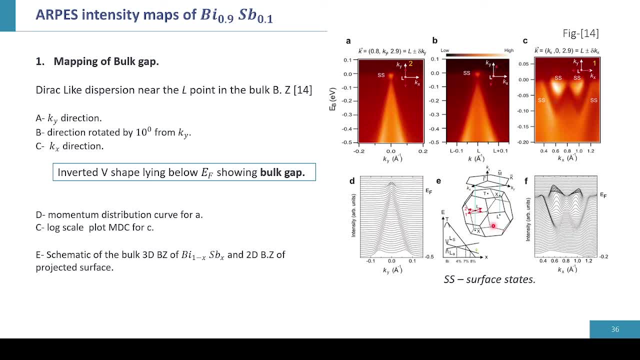 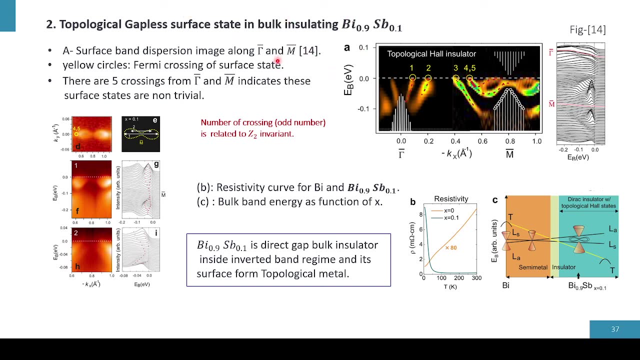 and this is how the 3d uh global zone of this with antibody alloy looks like. it is 2d global zone and this is the projection for the 2d case. now how would it be measured? that was the bulk state, and now for the surface state. we can see here the dispersion images along the gamma point. 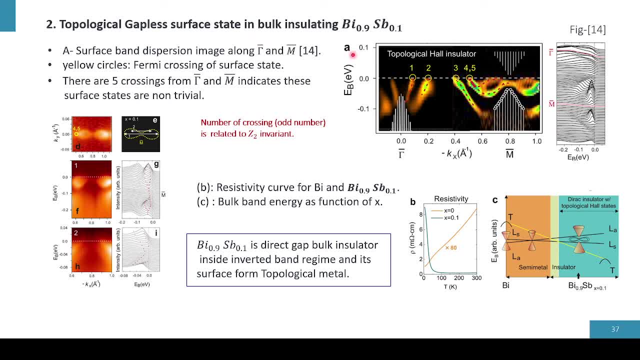 and the m dash point. that is the 2d uh projected one. so you can see the here. the circled one correspond to the fermi energy crossing. energy crossing is happening. that means the surface states have been created and this four and five are together. that shows that the two spins are there. spin up and speed. 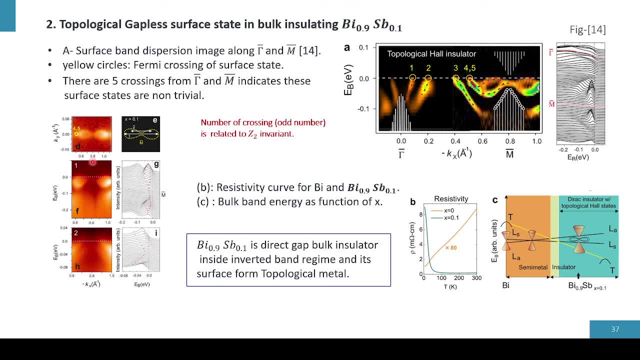 up that it is there. so this is assumed image of the uh energy crossing, which proves that there is a surface state, and the conclusion that i can give you is that this, this antibody is direct band gap incinerator uh inside the inverted band gap region and 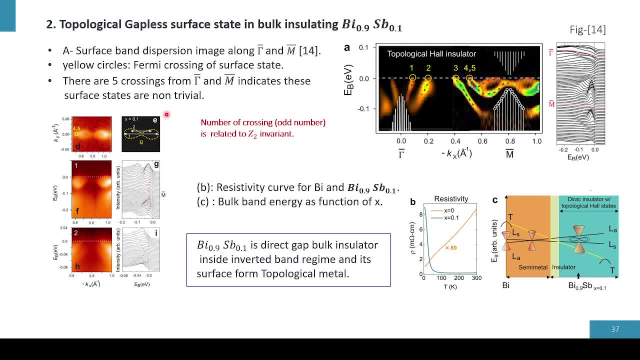 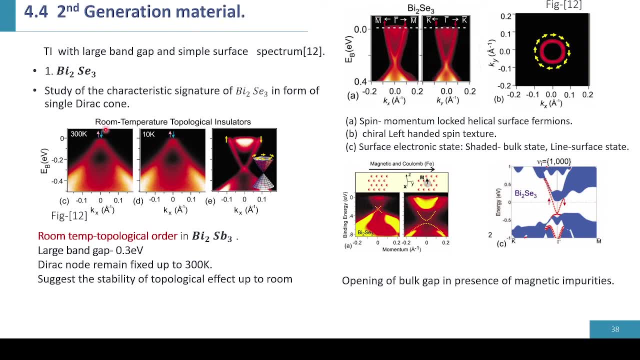 it is. it is topological material that conducting surface has a conducting surface. now we have a second generation material. the second generation material is much more advanced, but the surface state of the previous month must pass a quite complicated. so that is, they studied some other materials and this saloon became one of it, and the special is that this is a room temperature. 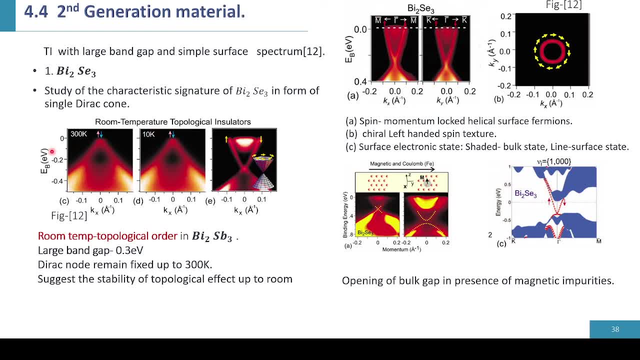 topological. so you can see they are increasing the temperature from 10 to 11 to 300 degrees can be, but still the single direction stays the same. that is robust, just not at all changing. and this is how the spin momentum. looking here you can see just the kind of left-handed spin. 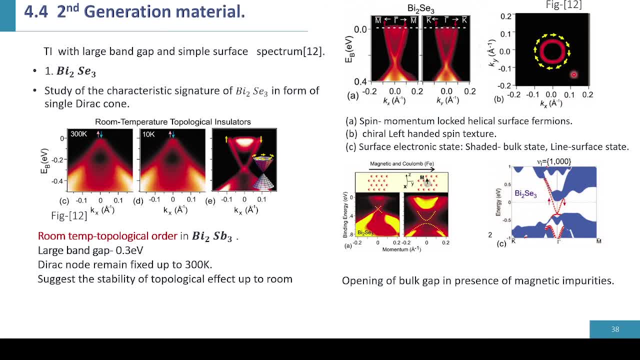 texture here and also important thing is that: uh, important thing is that in the presence of non-magnetic capability, as i explained before, uh in the 2d topological instead of it is robustly. similarly, here it is robust for non-magnetic impurities. you can see the 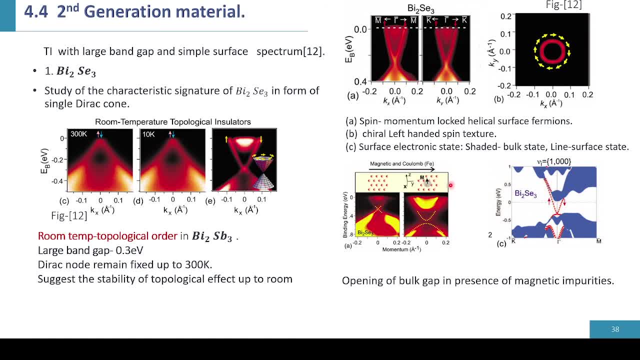 band crossing here. but in the presence of magnetic impurities like uh, iron, something like that, you can see the band gap formation. that means it is coming back to the insulates. we don't want that to happen, so that you're not to have a magnetic impurities inside, and this one is the energy. 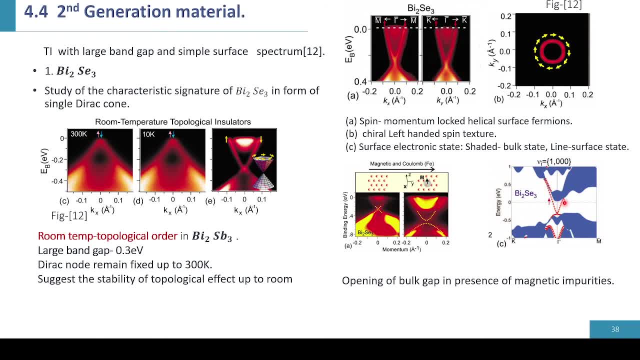 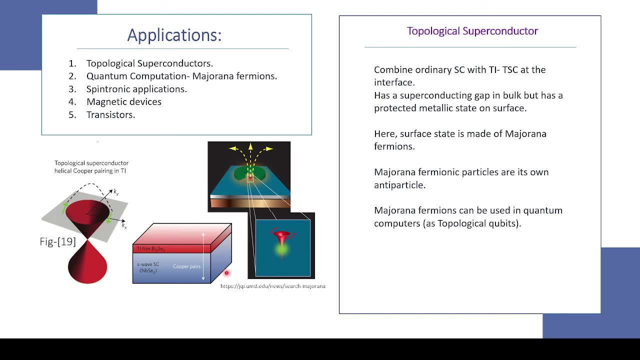 density surface. electronic state of density diagram. you can see the blue one correspond with the band state and this red one correspond to the head state. so that's the basic idea. so what are the applications? this has quite a good application. uh, as i told, this is one of the hot topics. 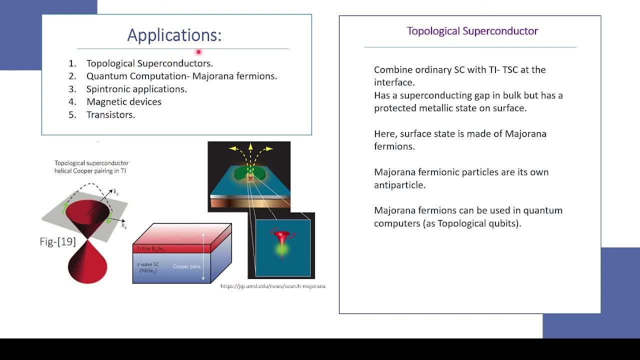 the applications are the topological superconductors, quantum computation, the. it is also applicable in spintronic devices, magnetic devices and also for making transistors. so when you combine, i'll just go through the topological superconductor, because that is a really hot topic now. so we combine the ordinary superconductor here. this can give uh. 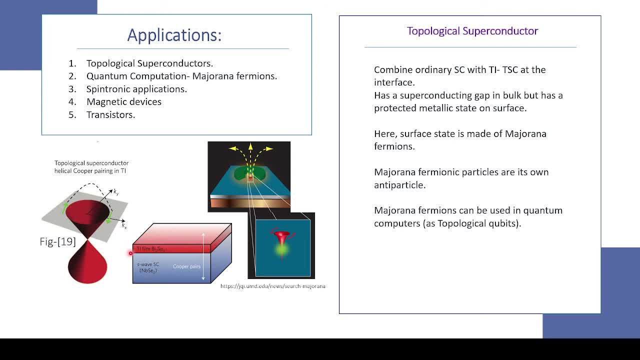 cylinder, and that is combined with the topological illustrator, the a2ac3. so instead of the copper cooper pair, formation to prepare formation will be there, but here inside the surface, in the surface, uh, so in the gap between them, the interface, actually the myeron of permeance, could be made possible. myeron of fermions is actually a particle which was 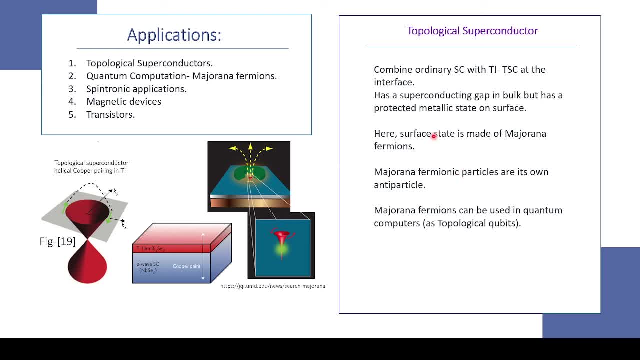 predicted by the hi-energy physics people and then now it is proven to be theoretically to be possibly found out, could be found out in the contest matter here, physics theory in this, topological superconductors. So anyway, Myronian fermions are particles which are its own antiparticles. So if we could detect, if we